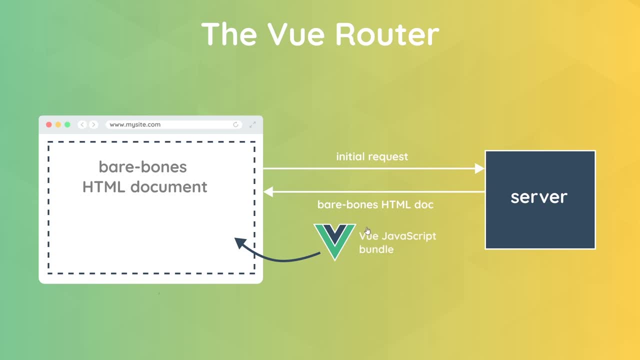 Then the server sends back an empty HTML document along with the Vue JavaScript bundle. Now Vue then mounts our Vue app to the DOM, the HTML page, so it takes the root app component and injects it into the HTML page. That's exactly what we've seen so far. 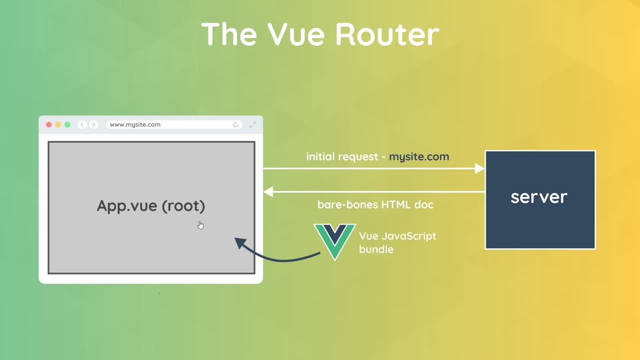 But when we also work with routing and the Vue router and pages in Vue, it takes one extra step. It looks at the route that we're currently on in the browser and then it decides what component to nest inside the app component dependent on that route. 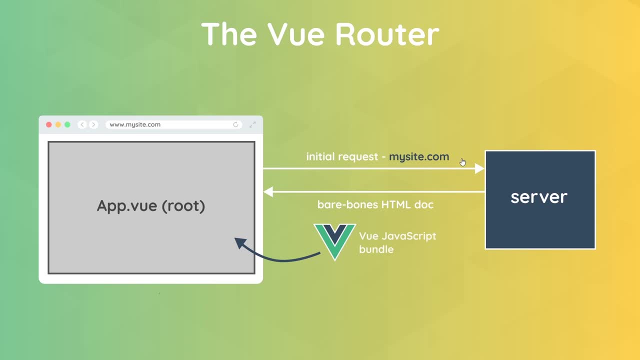 For example, in this case it will see the base route just forward slash because we've just gone to mysitecom, And in that case it might nest a home component inside the root app component. Now, if our initial request to the server was something else like forward slash contact instead, it would nest a contact component inside the browser initially instead. 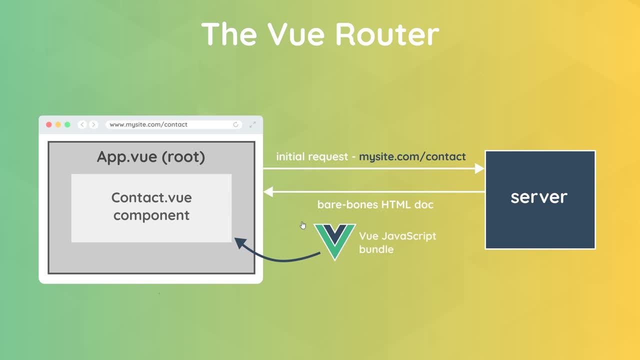 Now, thereafter, when we click links around the website, we don't send any more requests to the server. Instead, Vue intercepts the requests and looks at the route of the link we clicked. For example, it could be going to forward slash about, so it would unmount the current route component and instead nest an about component. 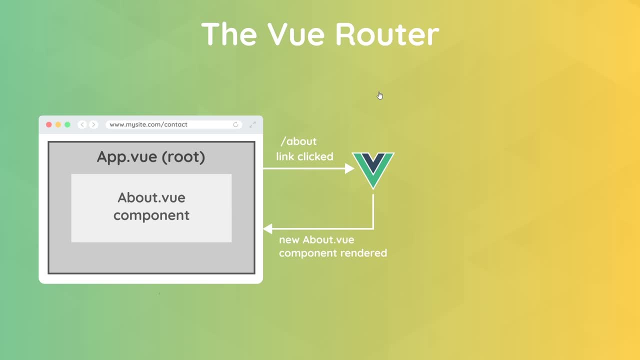 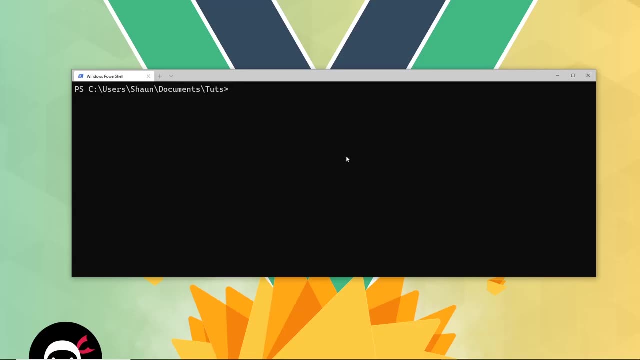 It's really simple to set up and once you get the hang of it, it will become second nature, And I'm going to show you how to set it up next. So in order to set up routing in our Vue applications, we also need to use another separate package called the Vue router. 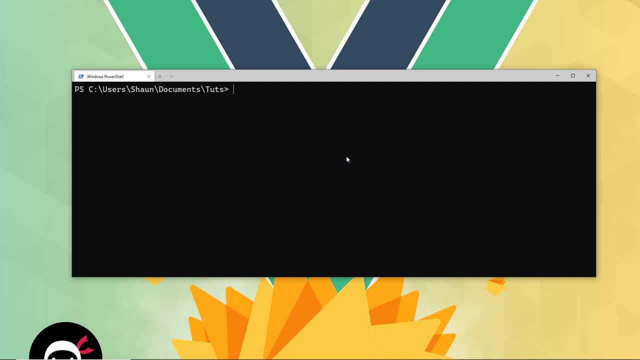 And the Vue router package works hand-in-hand with the core Vue library in order to allow us to set up a routing system, So you can do this manually in existing projects. You can. You can install the Vue router package and set it up yourself. 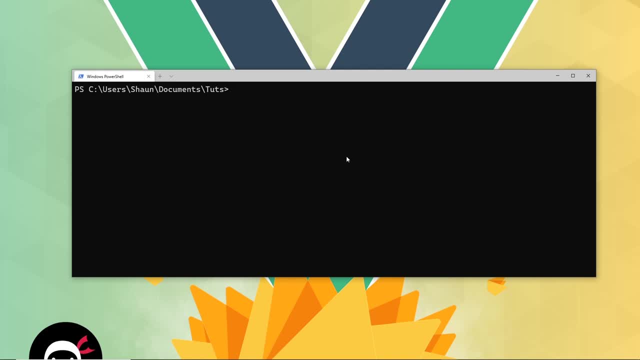 But the easiest way to get started with this is to generate a new Vue project using the Vue CLI and have the Vue CLI set up routing for us. So that's what we're going to do. I've already navigated to the directory. I want to create a new project in. 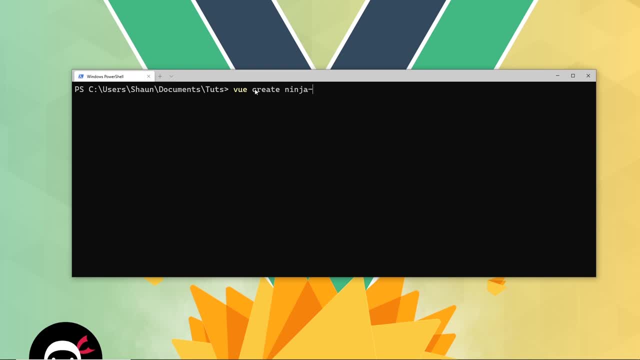 Then I'm going to say Vue create and the project name, which will be Ninja hyphen jobs. So we're just going to make a small project to demo this Vue router. So press enter to generate this project And we're going to manually select features. 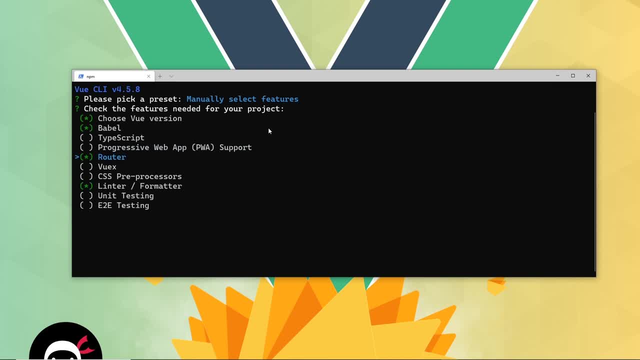 We're going to go down to router and press spacebar to say we want to install the Vue router and set that up as well. So the Vue CLI will then take care of all of that for us. I'm also going to unselect this and then press enter. 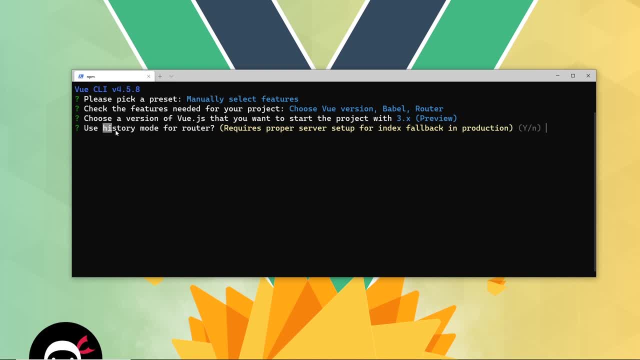 We'll use version three And this right here. this asks us: do we want to use history mode for the router Now? the other mode is hash mode, where we see hashes in our different URLs. We're going to use the history mode. 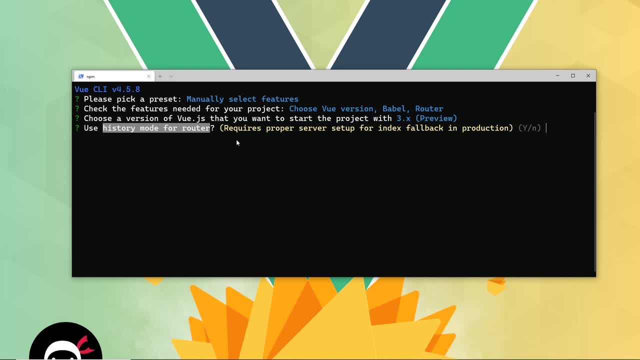 And this is more important- later when we come to deploy the application to Firebase. So I will talk about this a little bit more then. For now, just select, yes, the default option. We're going to choose default config file And we don't want to save this as a preset. 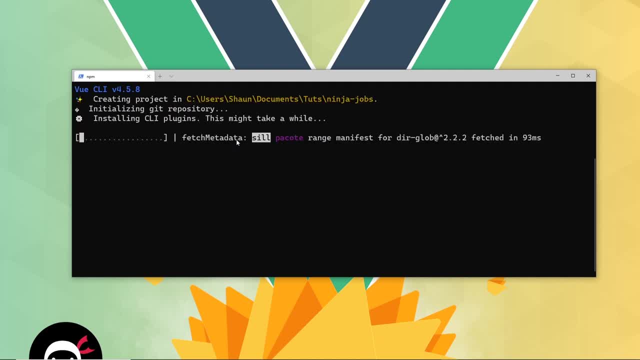 And then this will generate our Vue application for us. OK then. So once that's done, like always, I'm going to CD into the new project directory And I'm going to type in a name, which is going to be Ninja Jobs in this case. 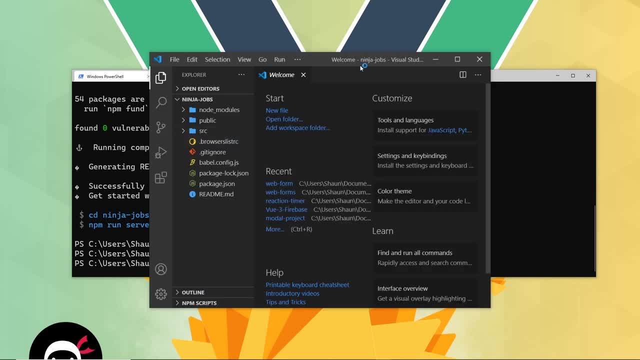 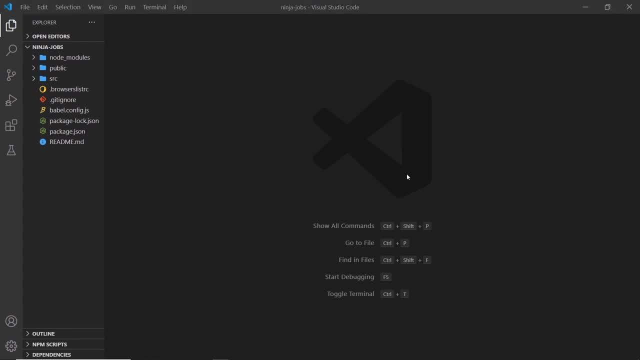 Press enter and then I'll type code space and then full stop. Press enter to open it up in Visual Studio code. And this is what the starter project looks like when we use the Vue router. So the first thing I want to show you inside this new boilerplate project is the packagejson file. 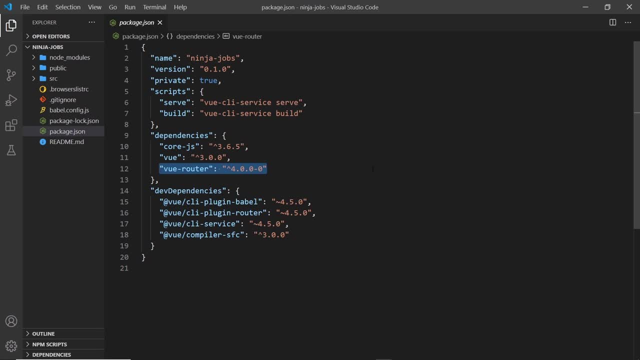 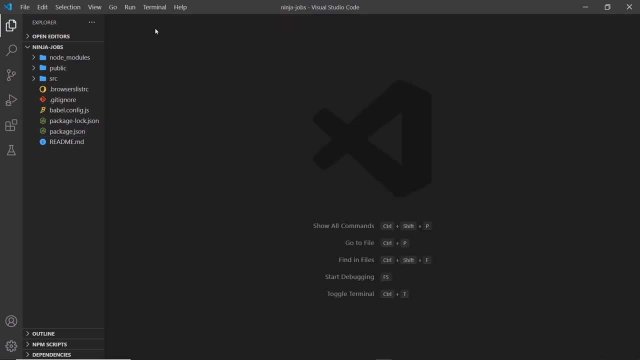 Because we now have a new dependency. This is the Vue router package that is now installed into this project And therefore we can use it to generate different routes. first difference. the second difference is inside the source folder. you see, now we have this router. 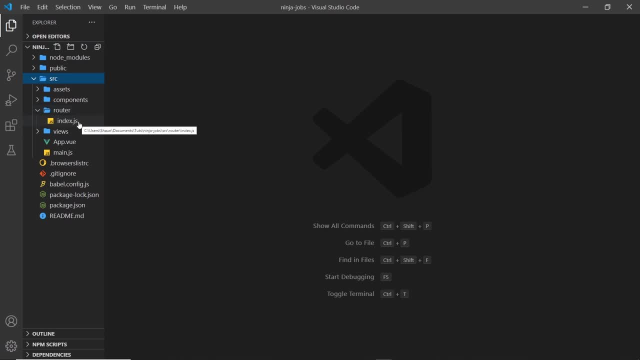 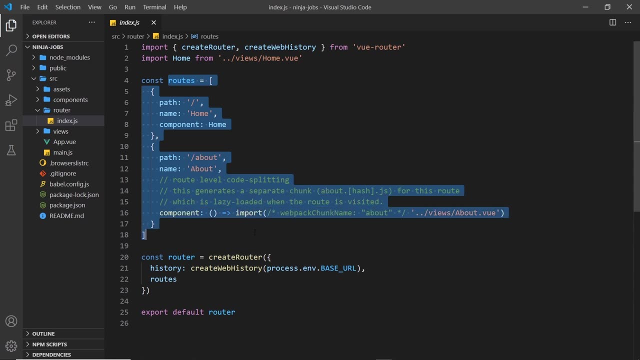 folder and inside that an index file that wasn't there before, and this is where we set up all of our different routes. so you can see, right here we have a routes array and this array contains different objects and each object represents a single route. so each route object has these three. 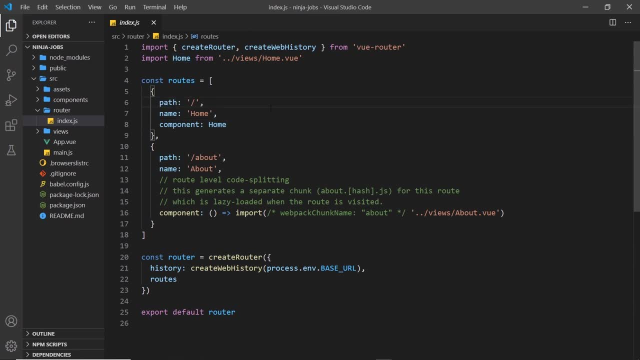 different properties. we have the path property, which is the url path relative to the root of the site, so in this case, just forward slash. we have a name property, which is a name of the route, kind of like an identifier. we also have the component that we want to use when a user goes. 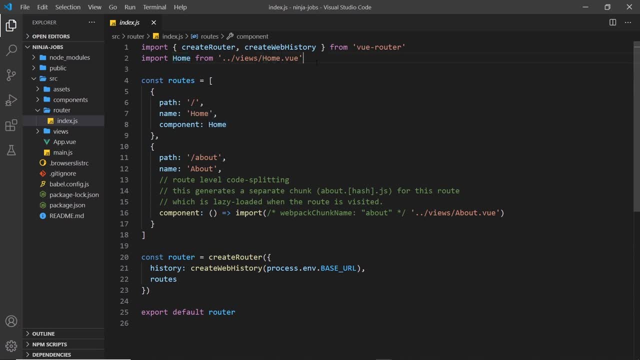 to this route and in this case it's the home component and that is being imported at the top. so that is a single route object. we also have another down here. the path is forward slash about the name. app has four routes, so those obj asses are there all now. these are all이에요 objects. 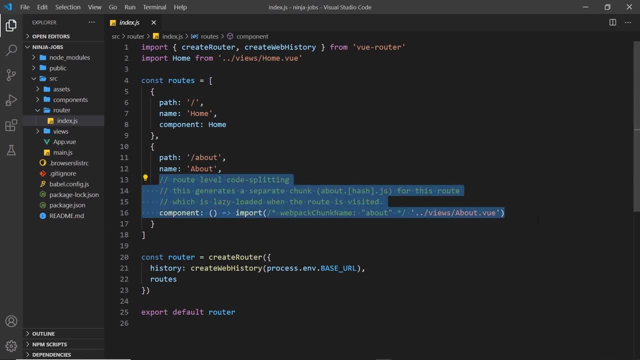 and that is being imported at the top. so that is a single round object. we also have another down here name is about, and this right here is showing you how to lazy load routes. I don't want you to worry about that for now. we'll talk about that later. for now, let's just register the components for. 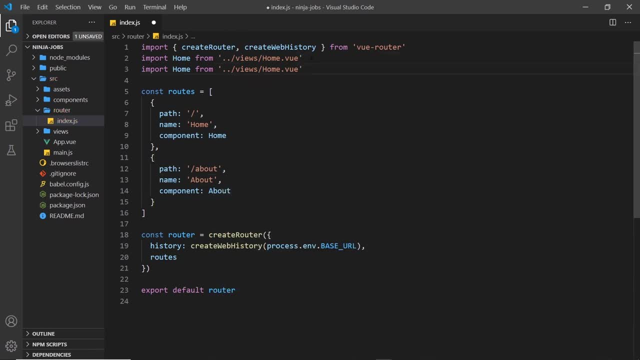 this route, which is about, but that does mean we have to import it at the top now. so let's change home to about. and now we have those components. I will talk about these later on, but for now we have our array now of different routes, but at the minute that is just an array and it's not. 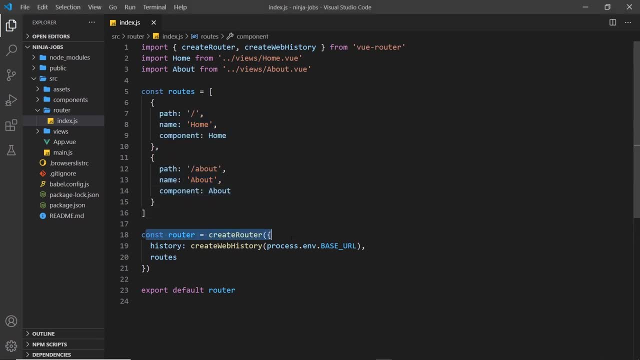 really doing anything. at the bottom of this file is where we actually set up the router instance. now this is the thing that actually creates our router for the app, and this function right here is being imported at the top from the View router package. now, inside that, we pass an object with a. 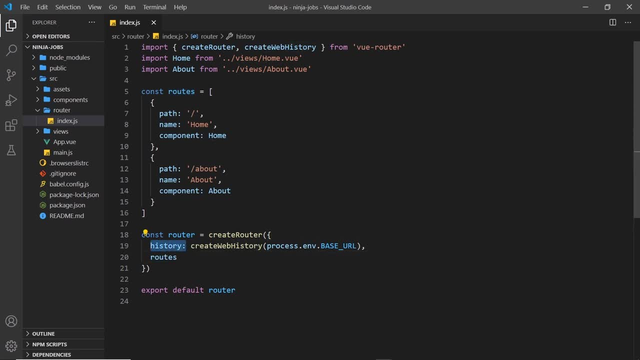 couple of different properties. the first one is the history property. now this function right here. create web history is saying, use the web history api in the browser so that we can click forward and back in our browser to go to previous routes. there's also a web hash history mode which places hashes in the urls, but we're going to stick with this one. 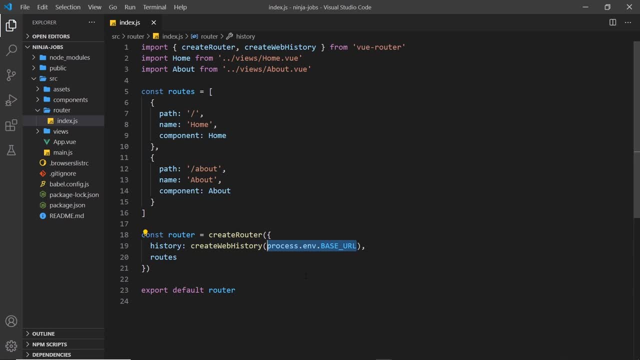 now, inside this method, inside this function, we also pass in the base url of our project. now, 99 of the time, you don't need to change any of the setup inside this router, but we will be changing our routes as we go forward. now the second property it passes in is the route itself. 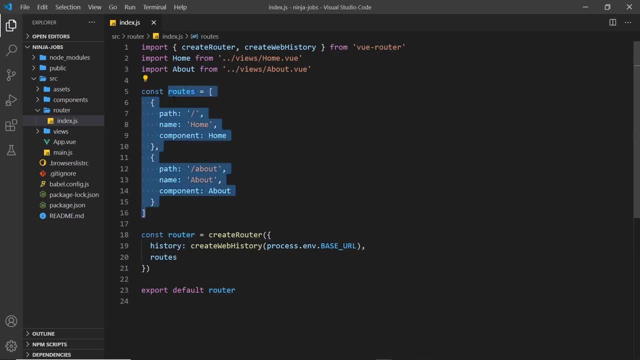 and that's so. our router is aware of the routes that we're using and it can register them. and then, finally, we export the router at the bottom. so whenever you want to create a new route, all you need to do is add a new object into this routes array. so this router, now that we export, 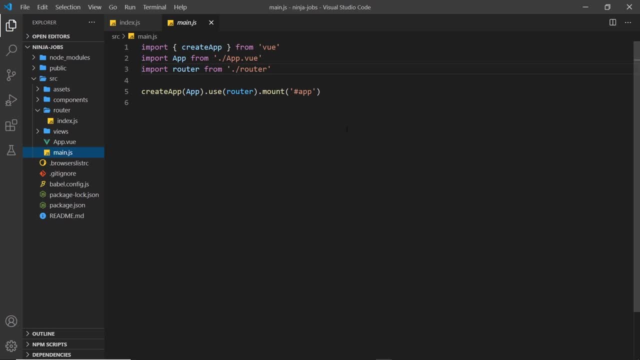 at the bottom is being used inside the mainjs file, where we kickstart the app and we're still using create app to create an application and passing the root component- the app- and we still mount it to the dom in the same location, but this time between those two. 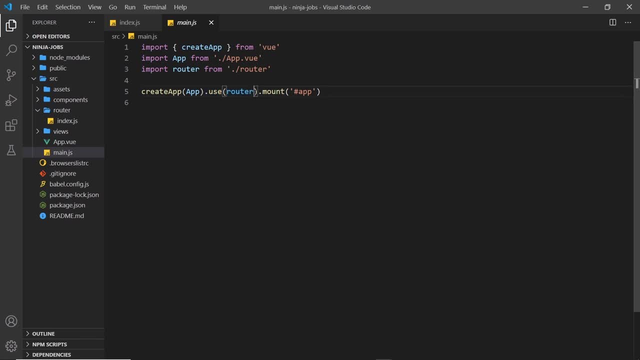 steps. we use this method, use, and this use method takes in an argument which is the router that we exported over here. so it imports that from that file and, by the way, we don't need forward slash index over here to import that. when you go to a folder and it contains an index file, it will. 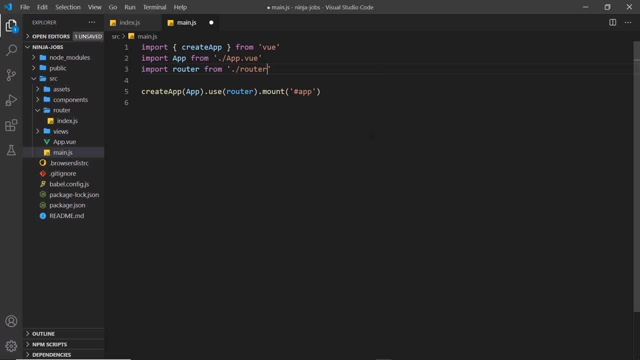 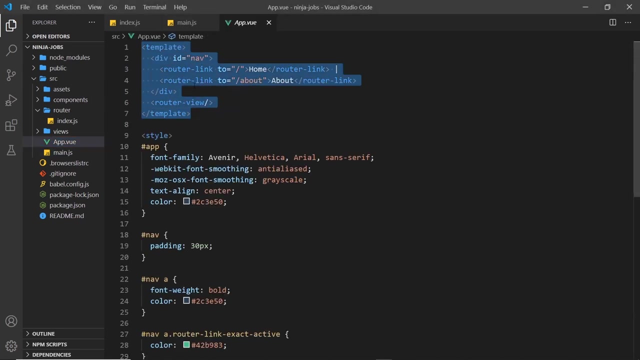 automatically import the index when you use the folder name. so we import that and we register it for the app right here. so now our application uses the router. that's what we're doing with the router object. but when we come to actually use our routes in the template, how do we set it up? well, if we go to app, view the root component and take a look inside, 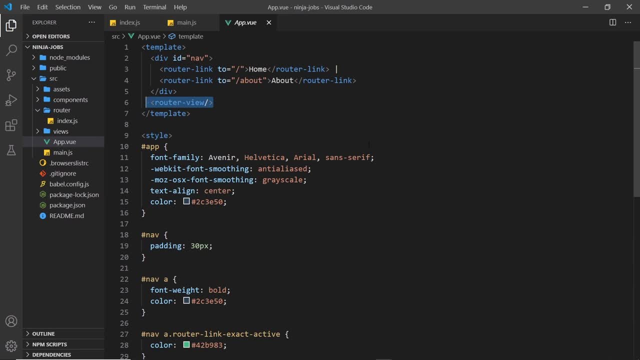 the template, we can see this router view tag right here. so this is router special tag that we can use without having to import anything. and right here where this tag is, that is where our route components will be dynamically injected, dependent on the route that we visit. so if i go to forward slash according to this, then i will get the home component and 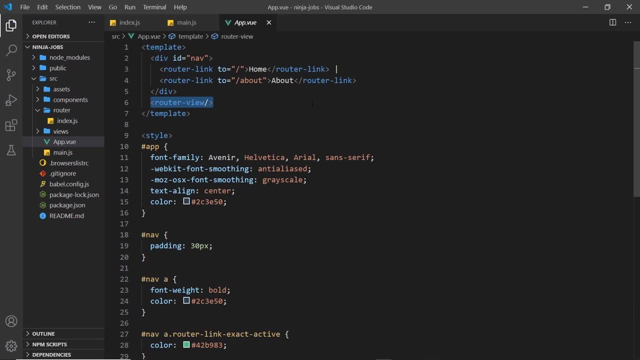 that home component will be rendered right here where the router view tag is. if i go to forward, slash about, then instead i will get the about component and that will be rendered right here. so that's how we use our route in the template and we only really need to nest this in the root. 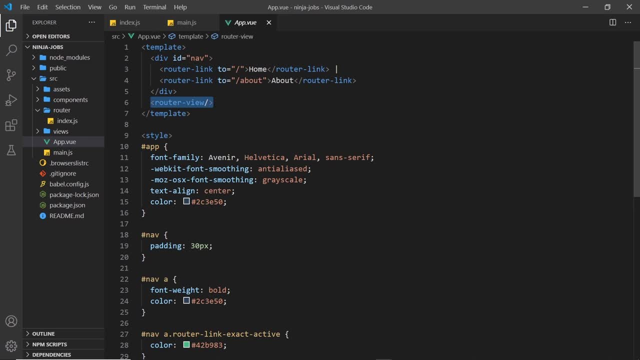 component and then whatever route we go to the component, for that route will be injected right here now. alongside that, we have a nav, and we could have something else like a footer below this as well. anything else around it. that will all appear on every single page, because it's not where the 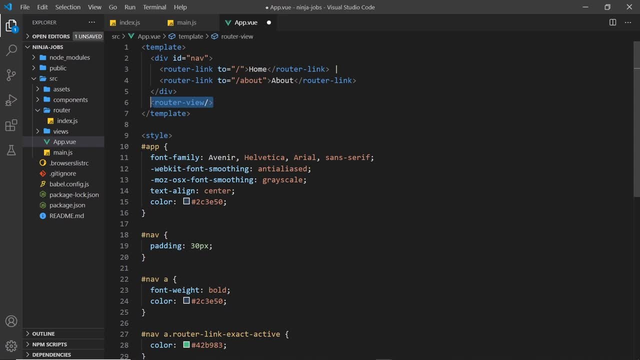 router view is. it's around it. it's only the different route components that will change where it should be. but if we were to go to our template and we were to go to this one, we could we go to different routes. now notice also this views folder right here now. this is where all of 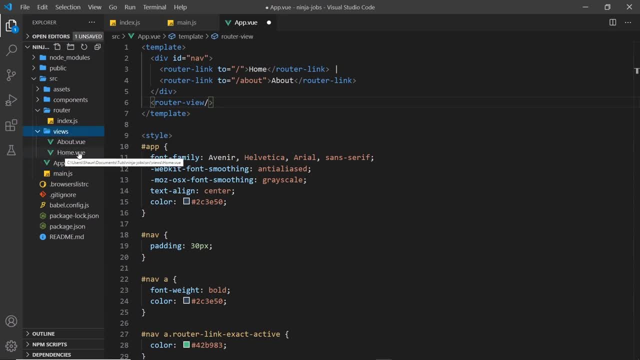 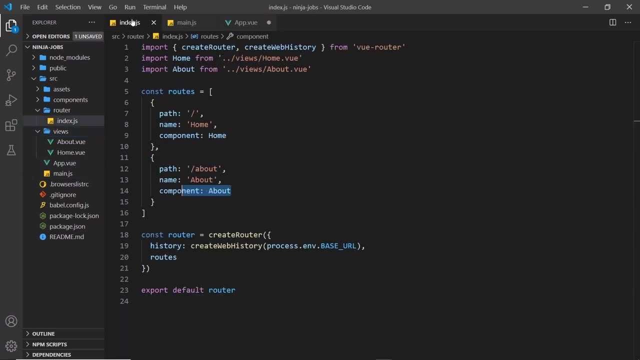 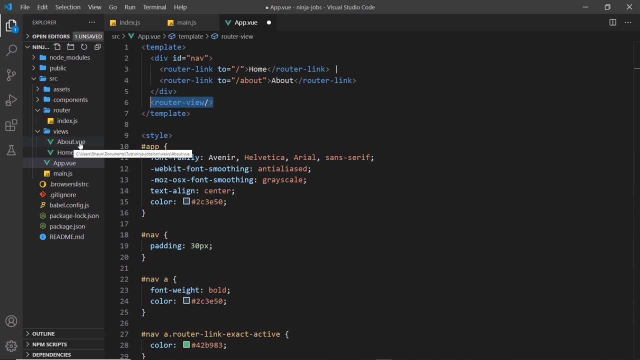 our different route components live, in our case the home component and the about component. so if we were to go to forward slash about because we registered inside the route file over here, forward slash about to use the about component. it will show this about component inside the views folder. 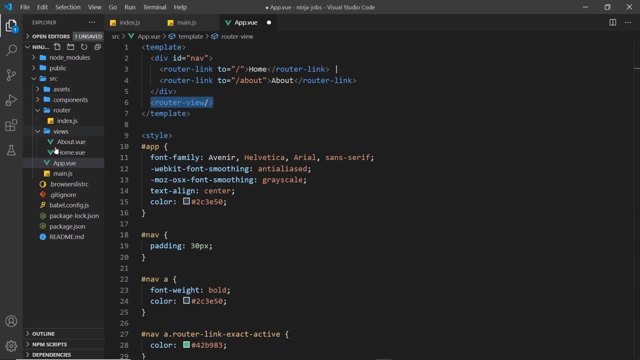 right here where the router view tag is now. we'll talk more about folder structure later on in the course, so don't worry too much about that for now. but we know now that our different route components are shown here, so i'm going to test all of this out in the browser. let me save this file. 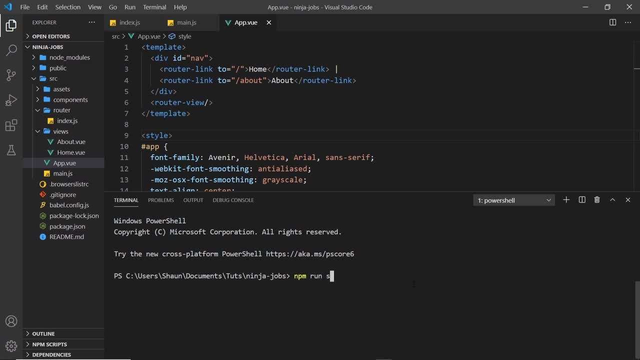 open up a terminal and then i'm going to say npm, run, serve. then i'm going to control, click that to open it up in a browser and we can see it right here so you can see it's set to route the view tag file in that folder here and then you can promote wakes. you can. 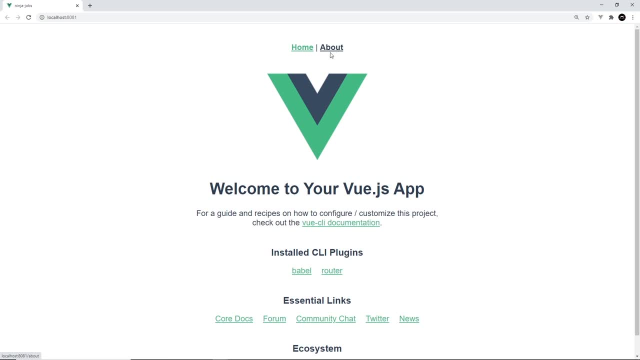 set humidity, set up from there, and you can use this to do the same for your impost. ね, we can remote. posso finish? see, we have this nav at the top and if we go to this and click on this it goes to forward. slash about and it loads in the about component. if we click on this, it goes back to the home page. 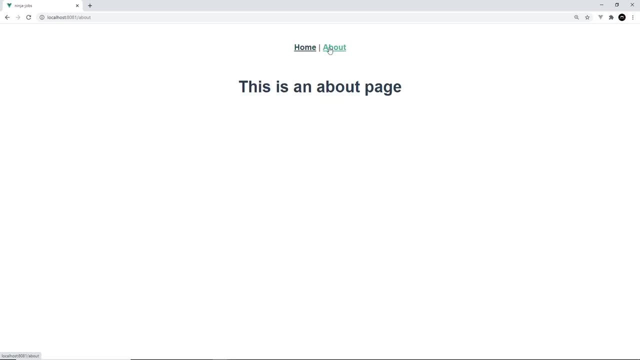 so notice how quick all of this is. it loads these different routes really quickly and we can also see the route change up in the address bar right here now. the reason it loads really quickly is because view is only switching out the components for different routes. a new request is not being. 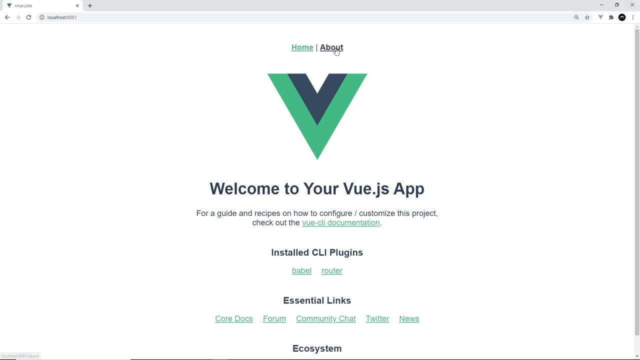 sent to the server for every new page, every time we click on one of these links. remember, when we first make a request to the server, it responds with just the bare bones indexhtml file and the bundled view javascript code. whatever the first request route is, view will look at that and inject. 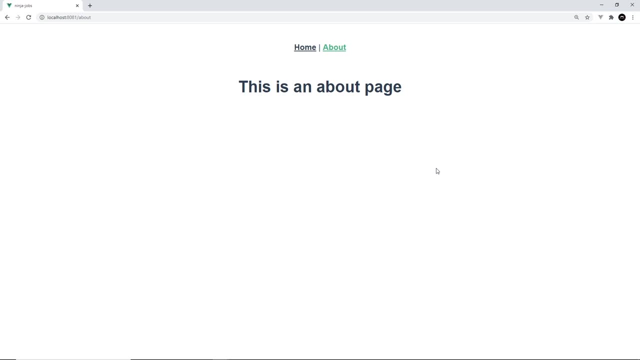 the correct components for that route into the appview file. for example, if the initial request is forward, slash about: if we hit enter, it sends back that blank html page. view will look at the route and it will send back that blank html page. if we hit enter, it sends back that blank html page. 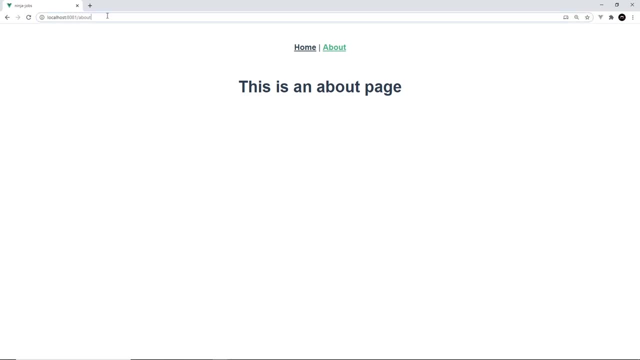 route and it will inject the about component because of this route here into the appview root component where the router view tag is now thereafter, any time we navigate around the website by clicking these different links, view is going to intercept the request for the new route and then it. 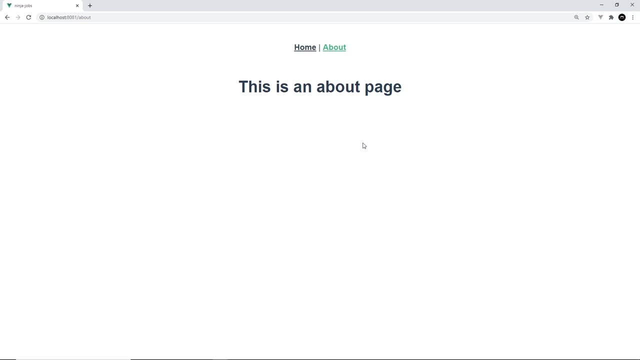 will look at that requested route and swap in the relevant components into the appview file. so all of the routing is done in the client, in the browser, and the requests for new pages are not sent to the server. and this is what makes the app much faster and slicker. now the way view does this intercepting. 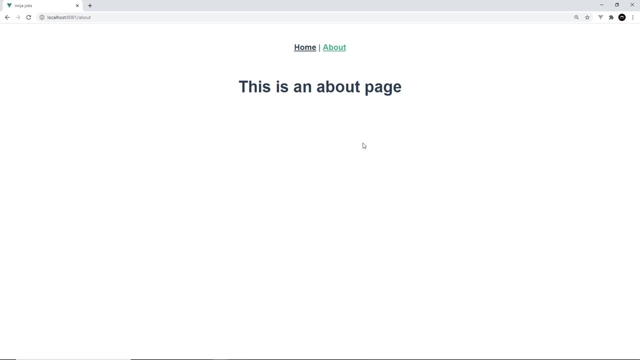 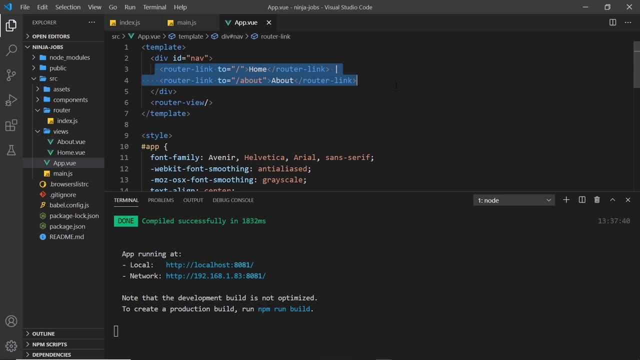 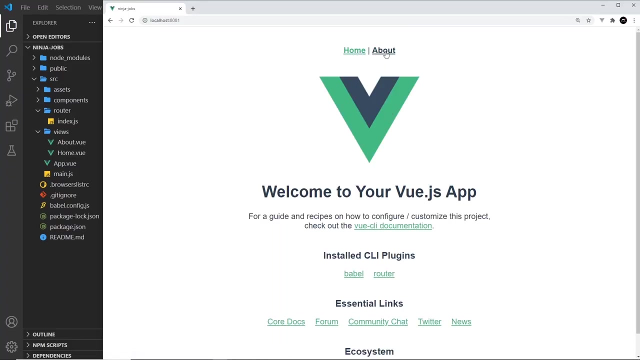 new page requests is by using a special tag called a router link, which, if we minimize this, we can see right here, and we'll talk more about those in the next lecture. okay, then, so we've seen how, when we click on these links, view intercepts the requests to get those new routes and it just replaces the component for. 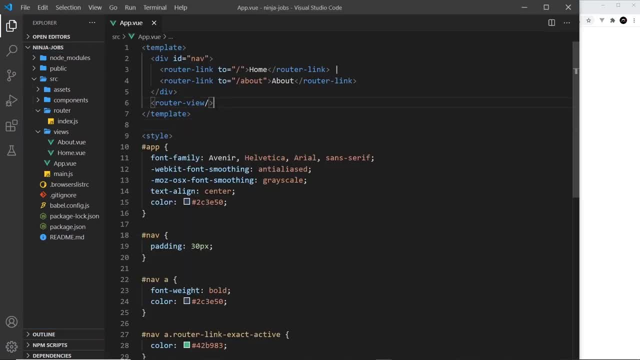 the page really quickly and that happens where this router view tag is now. the reason it can intercept those requests is because we're using a special tag and that is a view tag called router link. we're not using anchor tags right here now. this router link tag has a to attribute to say: 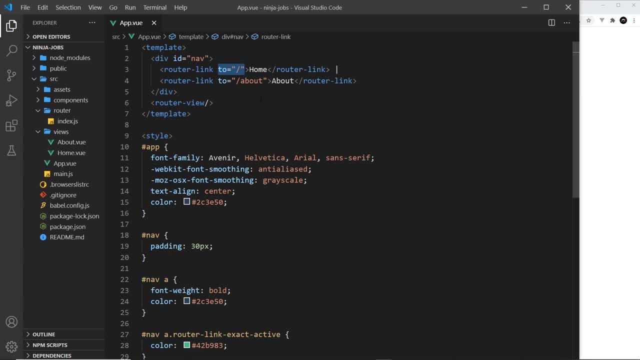 where we want to go to and that is the path and that's a bit like the href in an anchor tag. then we have some text and then we close off the router link. so this is the reason that view can intercept those requests, because we use these special tags with that behavior built into it. if 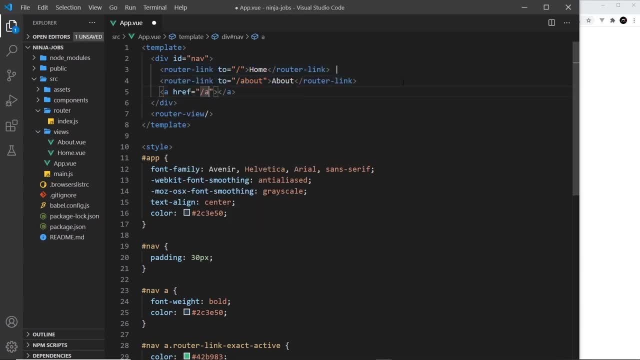 we were to use an anchor tag instead and say the href was forward slash about, for example, we'll say about right here, then this wouldn't work the same way, because this would just send a fresh request to the server and view would not intercept it because it doesn't have that. 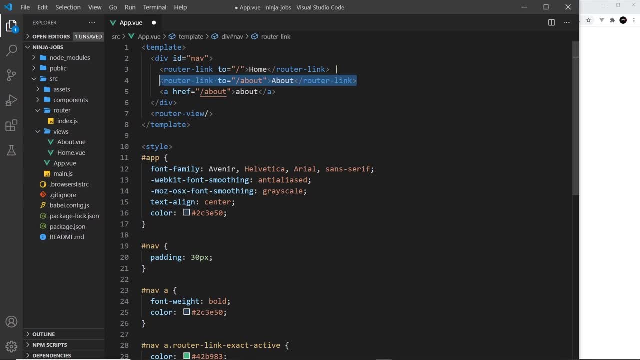 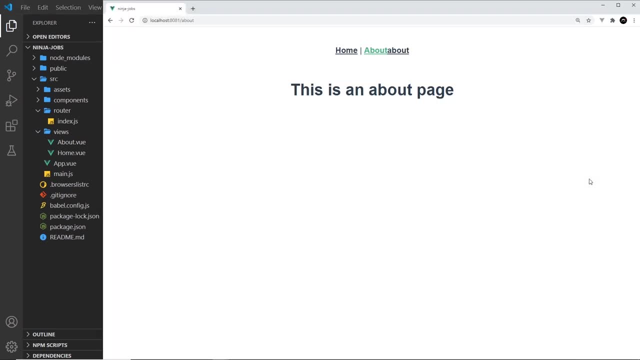 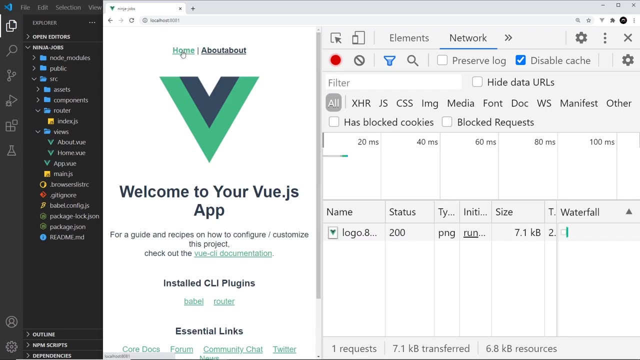 behavior built into it. this one has that behavior of intercepting the request built into it. i can demo this. let me come to the browser and open up the network tab, choose network and this is going to show any network requests. now, if i click on home, we don't. 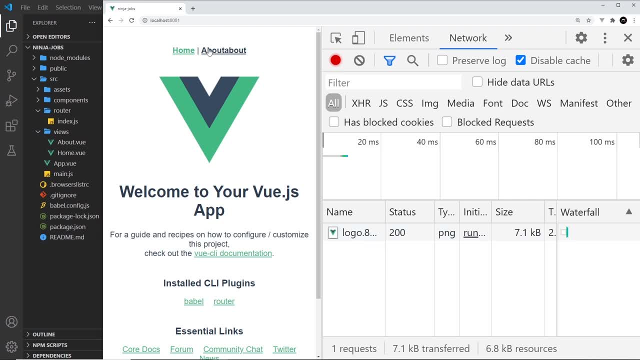 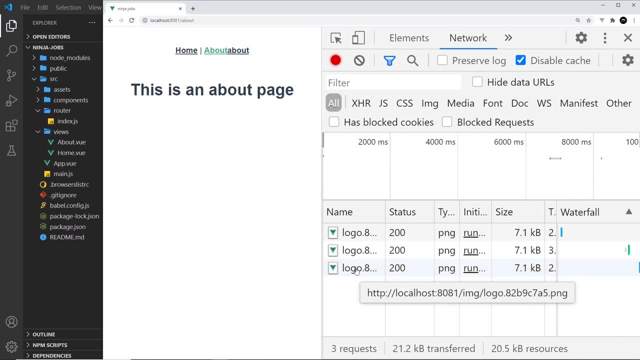 see a network request for another html page, only for the logo. if i go to about, we don't see a new one, and i can go back and forth and we only see network requests for this image right here, not new pages. now then if i click on this about one right here, notice we get all these new. 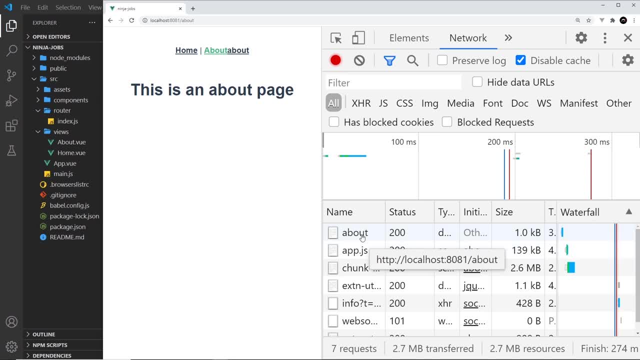 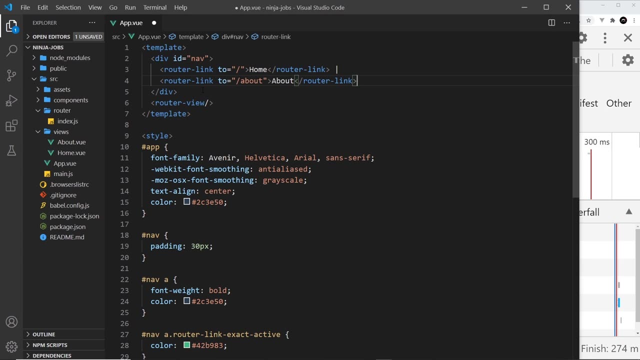 requests. one of them is going to be for an html page, one of them is going to be for appjs and other things as well. so view is not intercepting this thing, and that is why we use router links instead. that is much faster and it just changes the component rather than going to send a new. 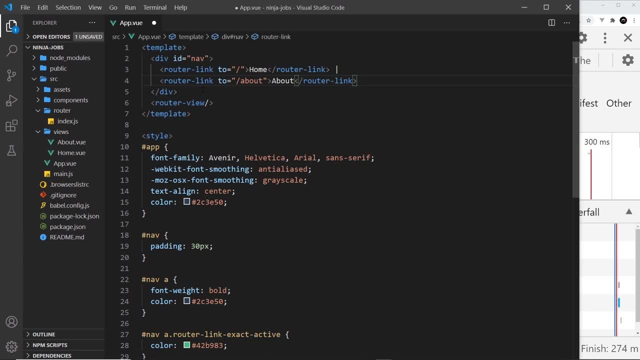 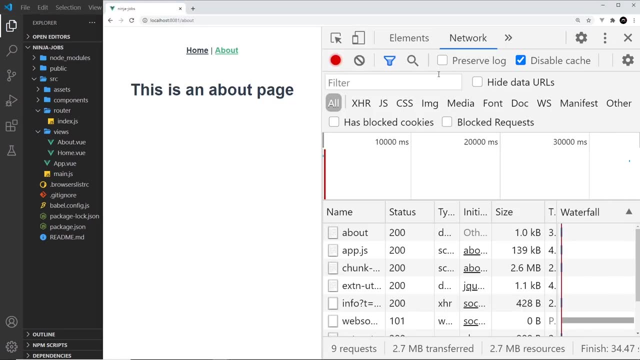 request to the server. now, as well as intercepting these requests, there's also other benefits to using router links as well. first of all, let me save this and head to the browser and i'm going to go to elements over here so we can see, and i'm going to inspect. 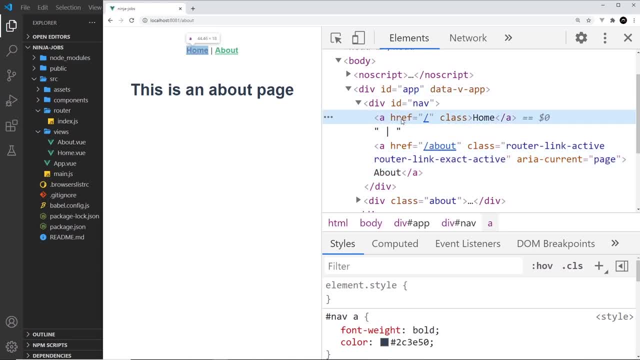 this one, and notice, by the way, when it renders to the dom. it is still just an anchor tag, but it has that built-in functionality under the hood. now notice, when we click on one of these, the active one becomes green, and that's because they get these classes automatically. you can. 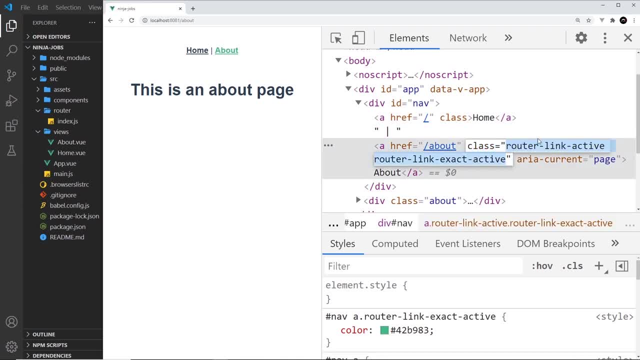 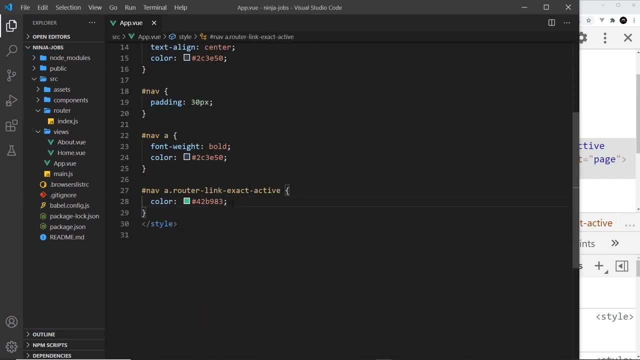 see router link active and router link exact active. okay, so we can style active classes or active links easily as well, and those styles are applied right here. now i'm just going to change this a little bit, just to customize it, and i'm going to say that the color of these 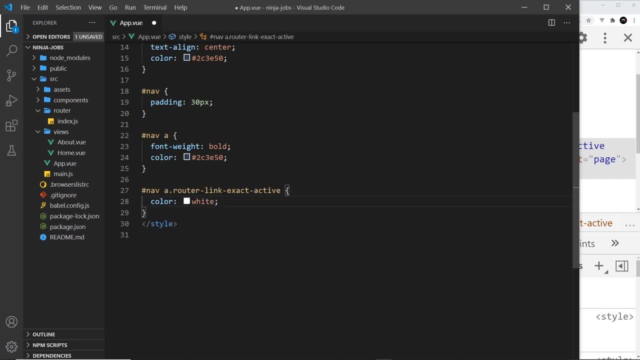 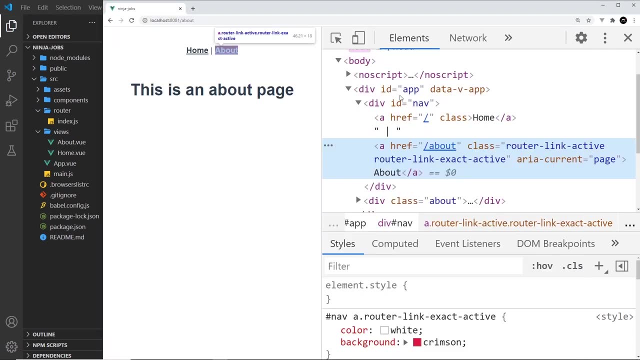 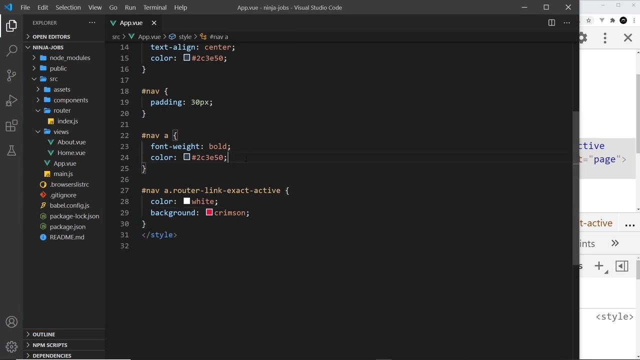 should be white and instead i'm going to apply a background of crimson like: so save that and preview, and now we can see that is the style of an active link. i also want to change this style a little bit, so nav a, we're going to say text decoration. 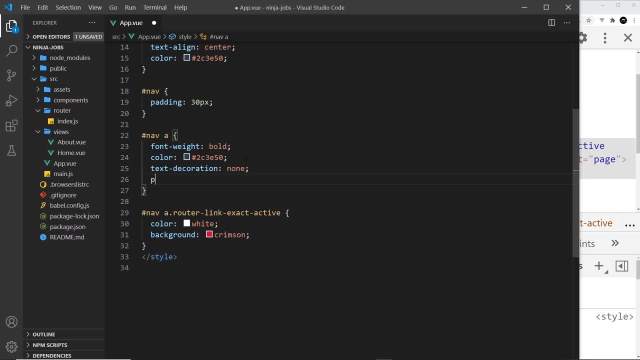 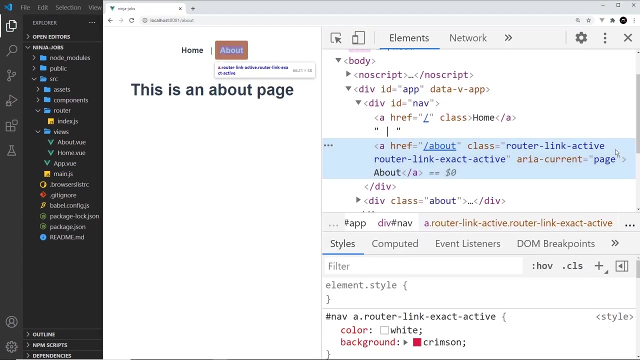 is none. so remove the underlining and then give it a bit of padding- 10 pixels- and then we'll also- oops, let me just change that to a colon- we'll also say: border radius is 4 pixels to soften the corners. check this out again, and cool, that looks pretty nice. so 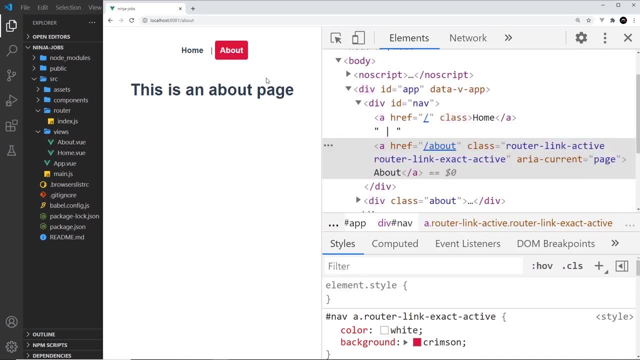 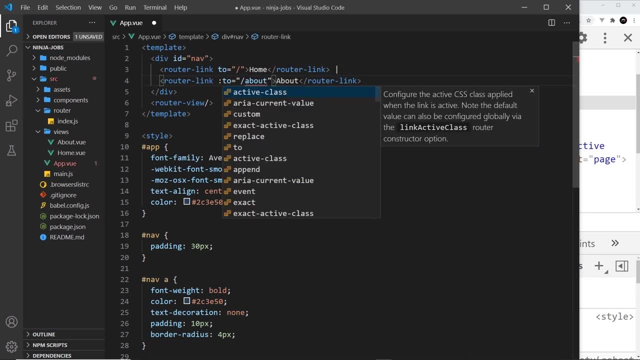 that is just another benefit of using router links. benefit of using these router links is that we can data bind to this two attribute right here, so i could say colon 2 and then, instead of hard coding the path right here, i could pass in an object which represents this route and then i could say the name of the route i want to go to. 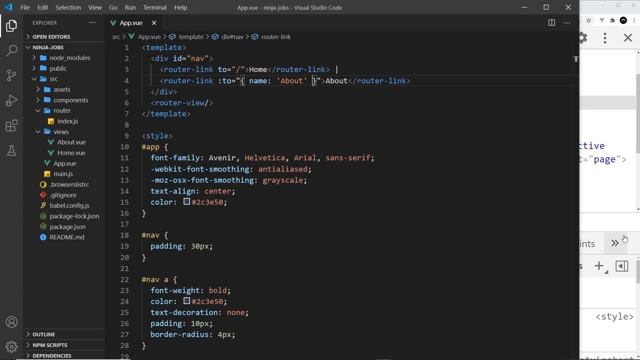 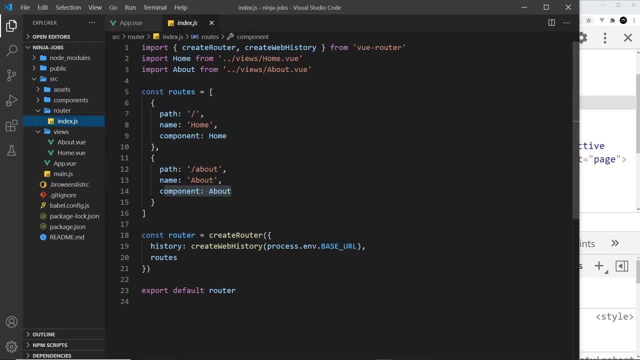 is about now. this is going to work exactly the same way because it's going to look at this object and see that the name is about. and if we take a look at our router file, we have a name property right here, so it matches against whatever name we place here and it uses that component. 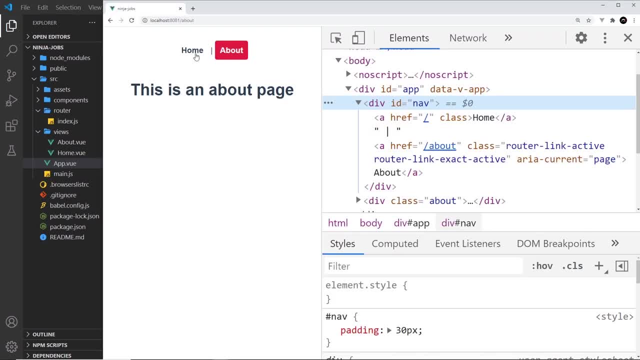 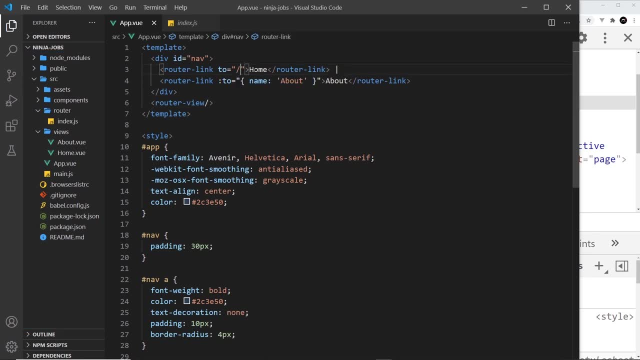 so what's the benefit of this? it works the same way, and i'm going to show you this. if i click these, it still works the same way. but what's the benefit of using this? well, if you think about it, your routes, your paths might actually change over time. for example, you 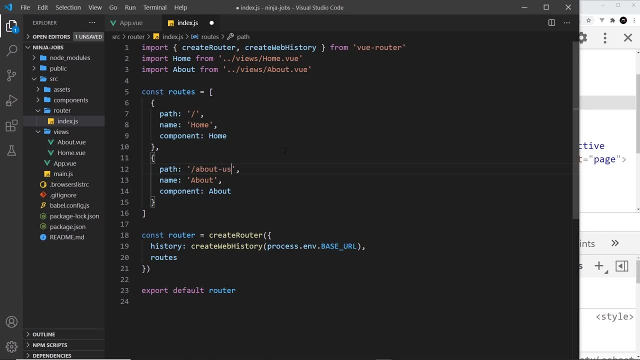 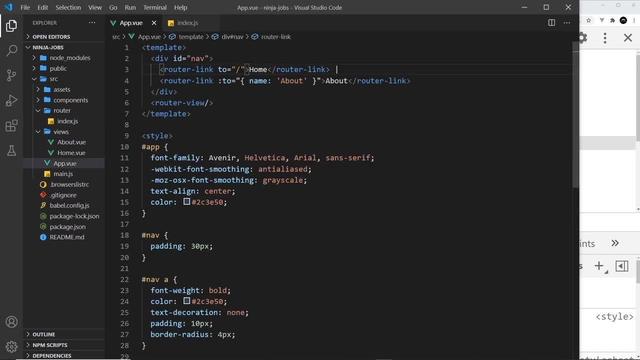 might decide in the future. well, actually it's not going to be about. it's going to be about us now. if that was the case, you'd have to go through the rest of your website and update all of your router links. if you coded them to forward, slash about and you'd update them. 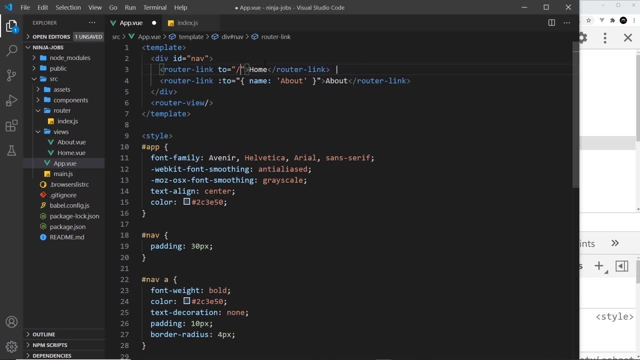 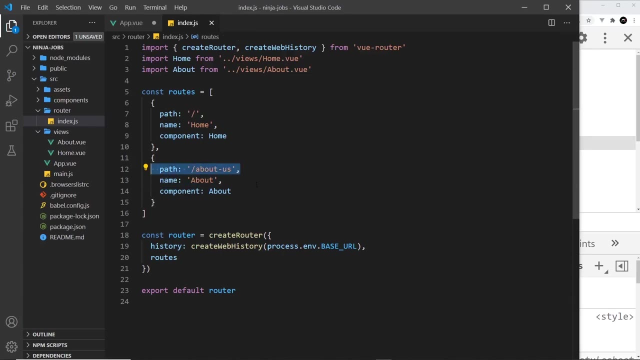 to about us. but if you don't use that way and you instead use this way of passing through an object and data binding to the two attribute, you don't need to change a thing, because it's still called the same name over here. it's still called about. it doesn't matter that this is changed, because we're 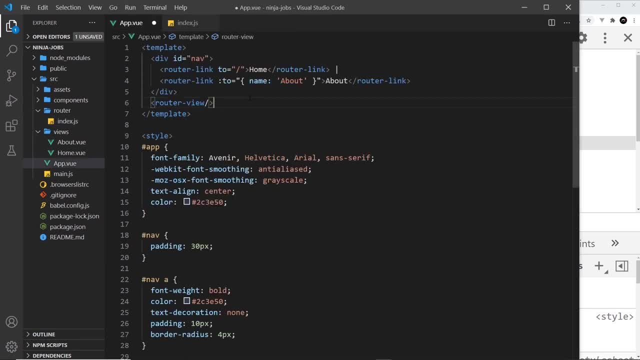 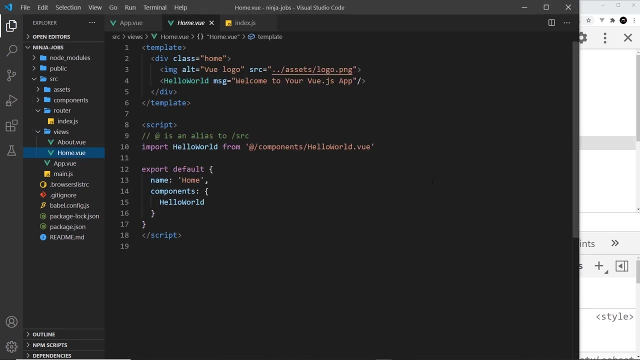 using the name instead now. so that's another way of using a router links and for the most part we'll have to go into the unknown and the council: um lorem ipsum, so paragraph tag and i'll say lorem and how many words i want, 100, press tab to create that and then duplicate it. so we've got a couple of 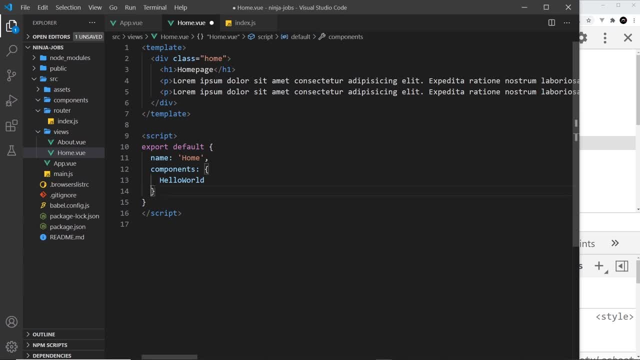 paragraphs right here of lorem ipsum. we can also remove hello world from the components right here. okay, so that's the home page, and if we go to the about page, i'm just going to add some lorem ipsum right here as well: lorem 100 tab and duplicate save that. 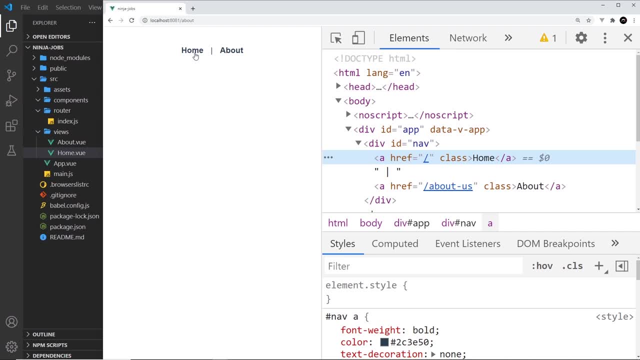 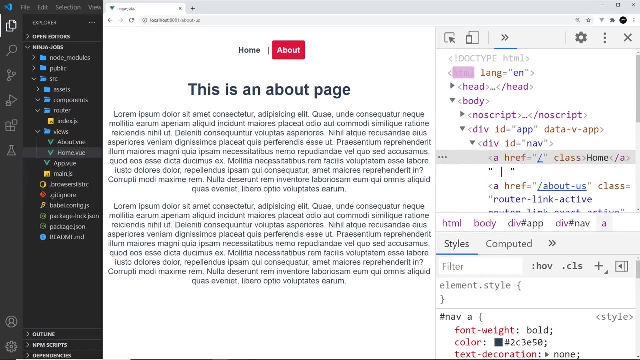 and let's view this in a browser. over here we have the home and we have about. now it's not picking up the change in content, so i'm going to hard refresh this page and now we see it and finally i'm just going to change the url back to about. 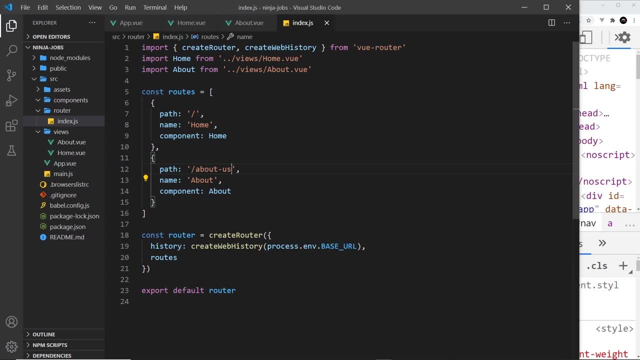 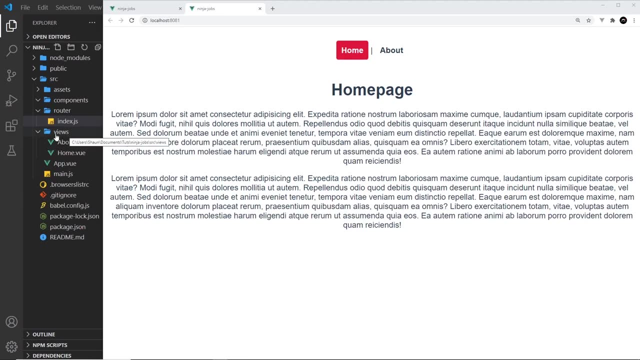 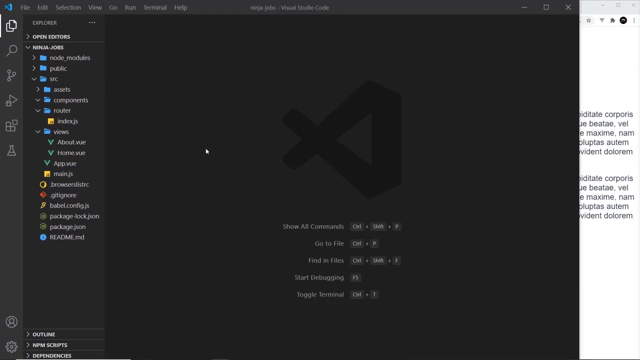 because i don't want it to be about us. so let's do that, save it, and that's pretty much everything for now. so next up i'm going to talk a little bit more about folder structure and this views folder right here in this lecture. i just want to take a few. 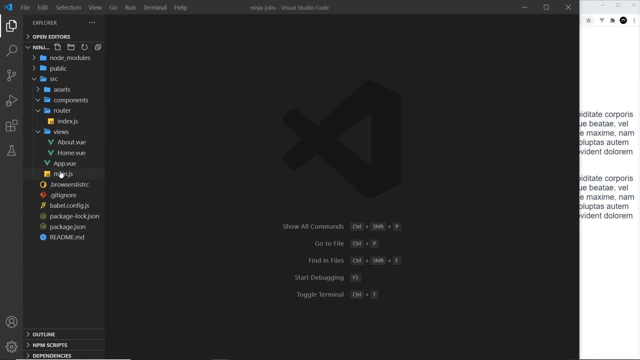 minutes to talk about folder and file structure and how you would organize your different components in these folders in a view application, because there's many different ways you can do this and how you structure your different folders and files is entirely up to you. i would just always 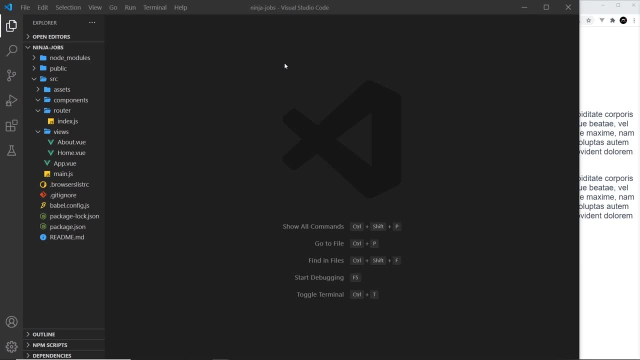 make sure it's constant and logical. now for smaller projects with just a handful of pages, i would tend to stick to this default setup where all of my route components are inside this views folder. so if i had another page like a contact page, i would make a contact view file. 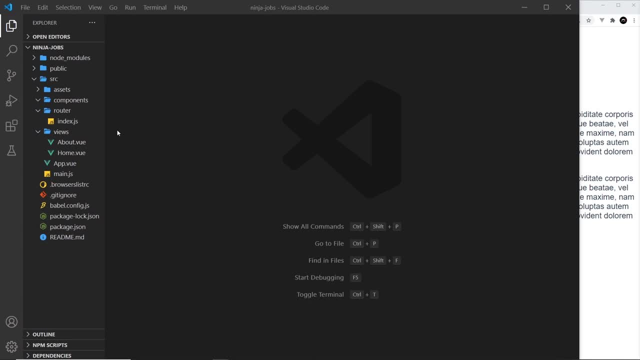 inside the views folder for it. now sometimes i'd also create subfolders for different pages as well, to group route components or sub components together where needed. for example, if i had a page which was a list of jobs, then i might create a jobs component first of all, like this: 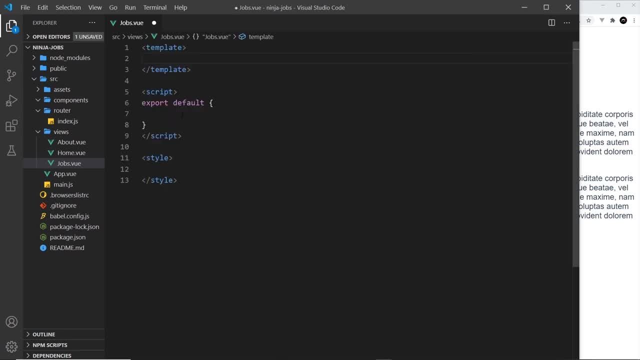 and let's just flesh out this component and inside the object down here we'll have some data and inside the data we need to return an object and i'm going to create a jobs property, which is an array of data. now i'm just going to paste. 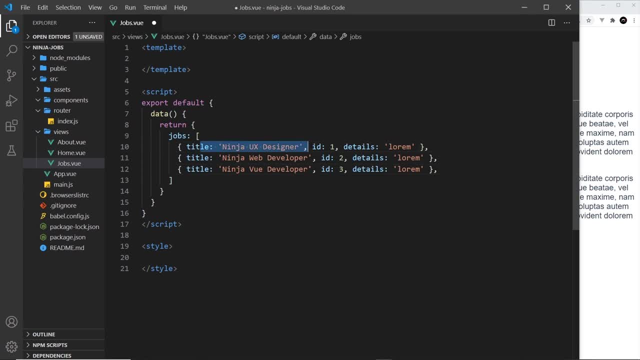 in three objects here. so we have a job title for each one and id and some details which are not very descriptive in this case. but we have some data and let's say we want to cycle through that data now. first of all let's do an h1 to say jobs, and then under that I'm going to cycle through the data. 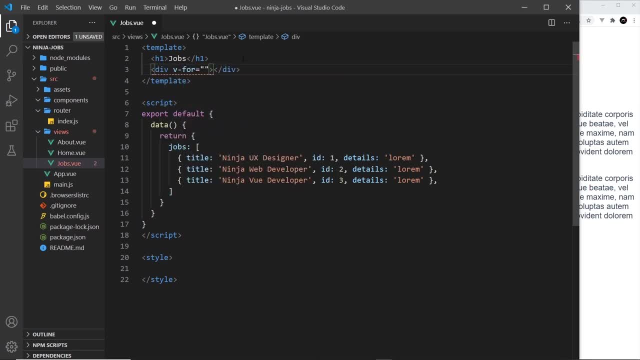 with a div and I'm going to say v-4 on this div and we're cycling through the jobs. so I'll call each individual job a job and say in jobs: remember, when we use v4, we need a key property which must be unique for each job, and that's why I created this ID property right here. so we'll set it equal. 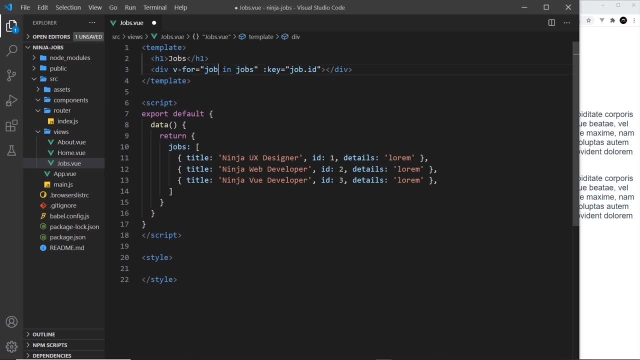 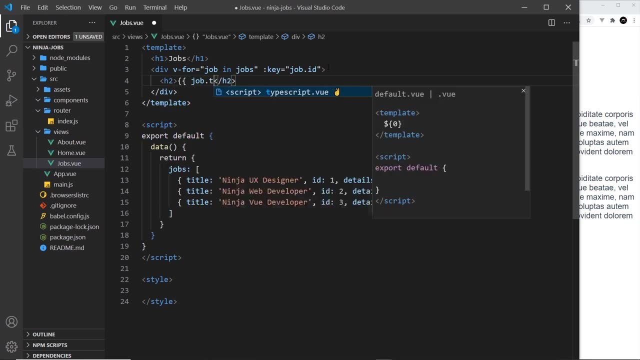 to jobid. we have access to job because we have it right here and then inside that, all I'm going to do is output the job title inside an h2, so job dot title. all right, so we have this component for the jobs page. we'd also need to register that route, so let's do that over here inside the oops. 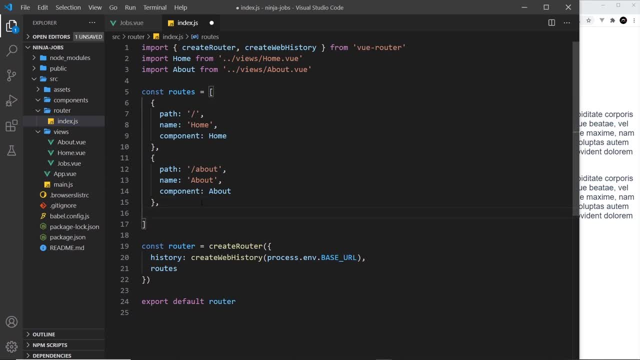 not that one, the indexjs file at the bottom. I'm going to create another object and I will say: path is forward, slash jobs and the name of this component is going to be jobs and the component we use is going to be jobs and we also need to import that at the top. so let me duplicate this and change about to jobs. 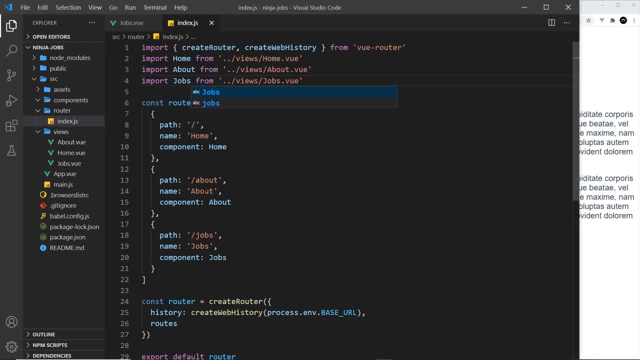 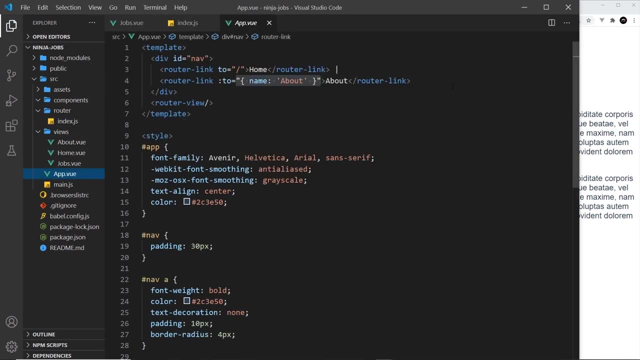 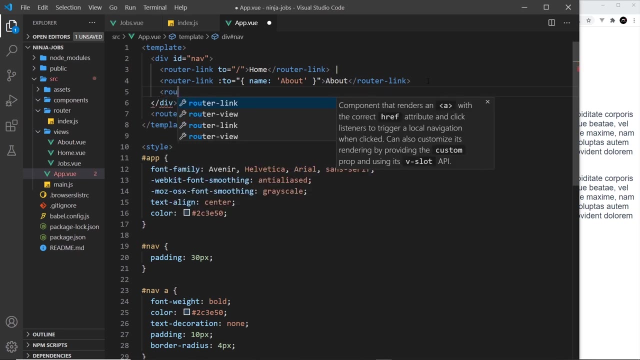 like so. now, if I save this and go to forward, slash jobs, I'm going to get this jobs component. before I do that, I'm going to go to the app component over here and I want to add now another link in the nav to go to the jobs page. so let me come down here and do another router link, like so, and then I need to. 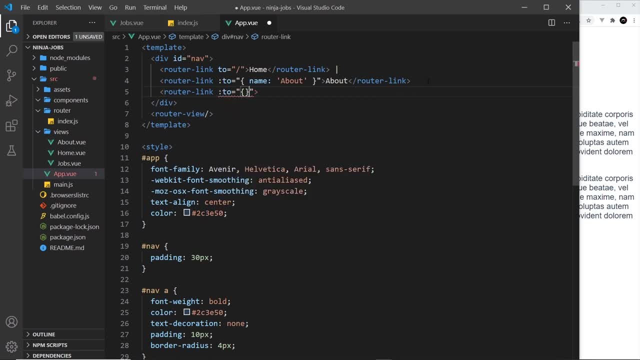 bind to the two attribute and set it equal to an object, because we're going to use this structure right here instead of using the path, and the name of the route is jobs. that's what I called it inside this file right here. so I want this to say jobs. and then we need to close off that router link. 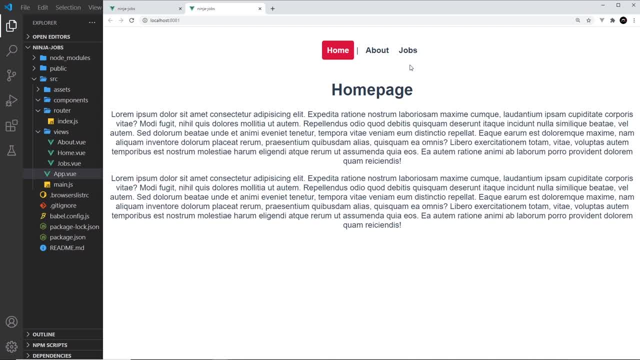 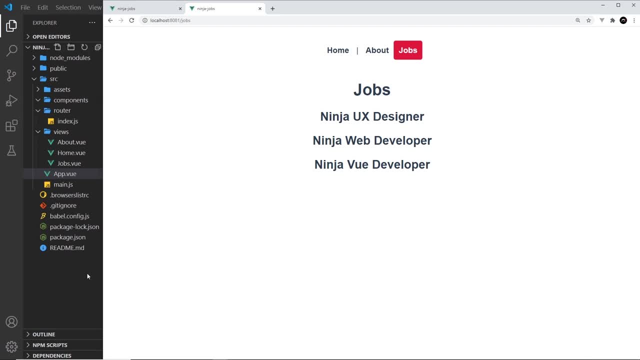 as well. okay, so if I save this and preview, we can see we have jobs over here as well, and if I click on this, we see all of those jobs. so all of that is working. but now let's get back to the folder structure. so imagine if we were to click on one of these jobs on the page. then we might link to a job. 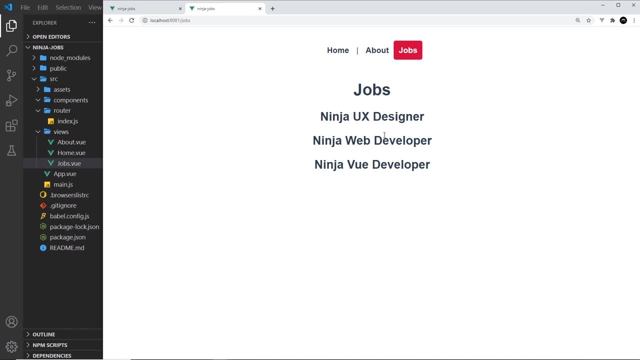 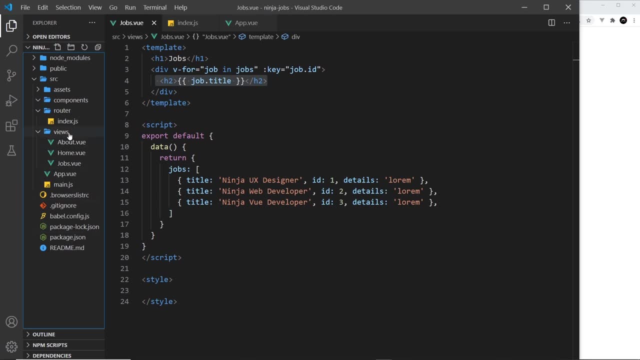 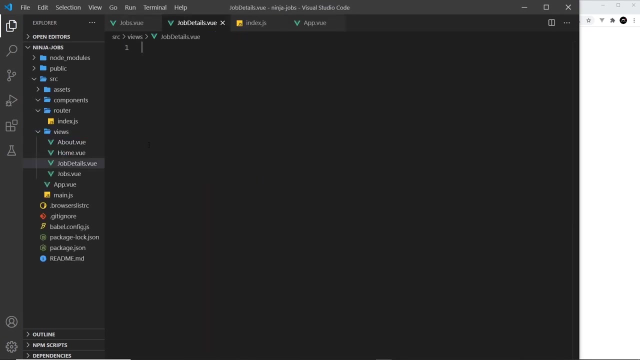 details route which would show a job details component and that would list details at that particular job. so we need a job details component, right, so we could create that in here like this job details dot view. now it's at this point I might consider creating a subfolder inside views, because this job details component and this jobs component 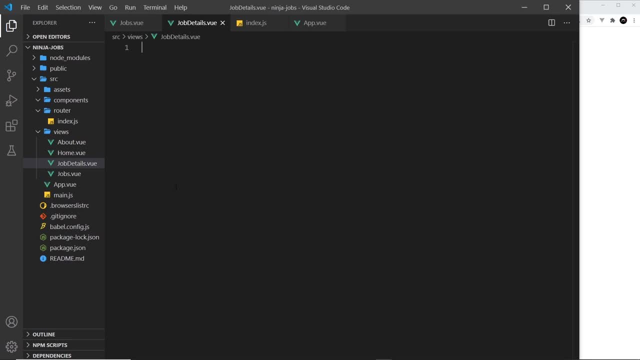 they're kind of related. they use the same data and they're going to be in the same kind of area on the website when it comes to URL structure, so I would probably create a new folder and call that jobs and then replace job. stop viewing there and job details in there. now notice: when I did that, I get an error. 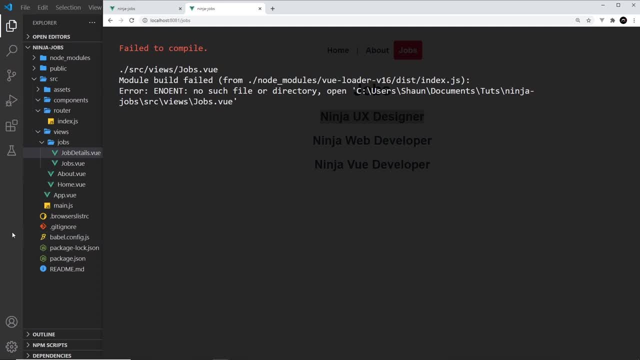 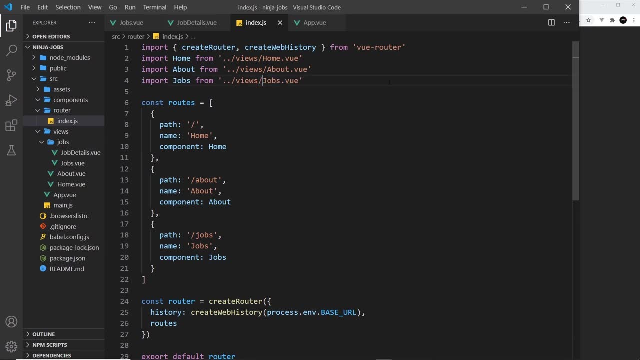 over here because it's not found that component inside the route file and that's because we're trying to import it from the top level of views. so we need to change this as well. so jobs and then forward, slash jobs, dot view and if we save that now, it should work. so this just makes our 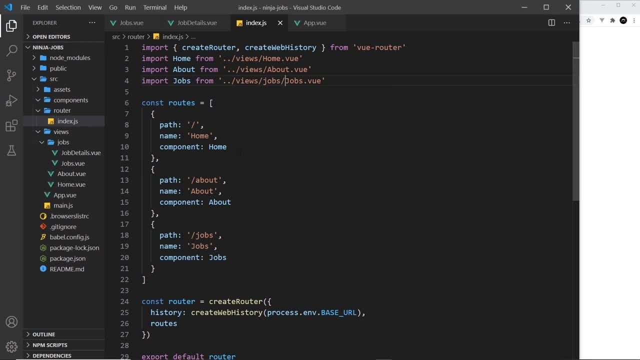 folder structure a little bit more organized, especially for larger sites with many different components and views, and this is the structure I'm mainly going to be using for routes or view components in the rest of this course also, I'll be using the components folder up here for any. 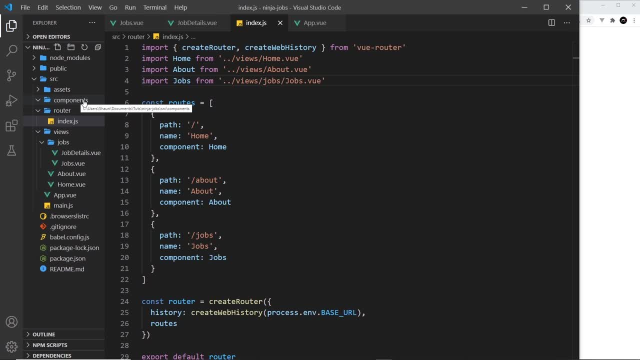 reusable components that can be nested into our view components. now these would be for things like models or custom button components that we make, or maybe a card component or anything else which really isn't page specific. it doesn't belong to a specific page and it can be used in a number of 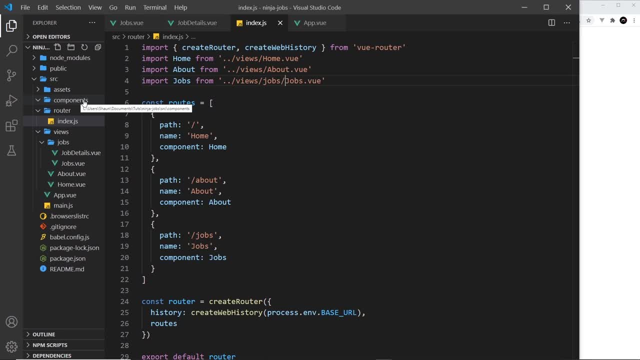 different views, so all those kind of reusable components will be going inside there and again. it may be at some point that we have subfolders for certain types of reusable components inside here as well. so that's it as far as folder structure goes. we'll talk more about the route. 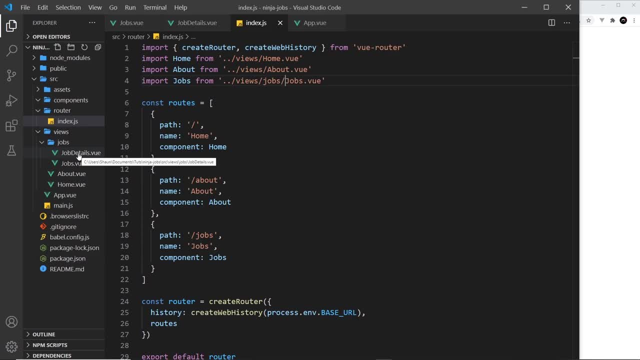 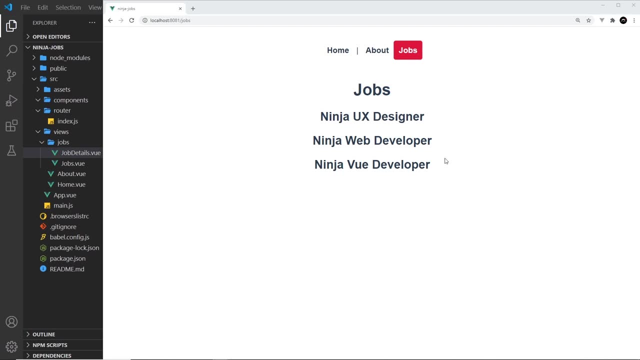 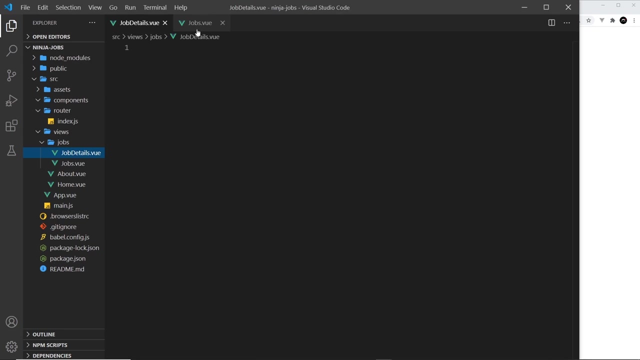 for the job details right here in the next lecture. so we have a jobs page and jobs component now which lists all the jobs and like to be able to click on a job to see a details page for that job. now we've already made a jobs details component, so we should show this component for that page and that route and so for each of. 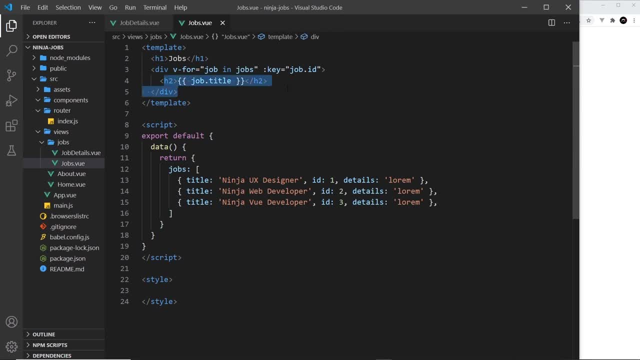 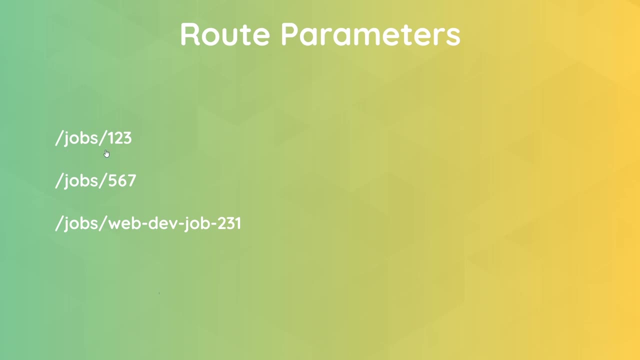 these jobs that we output inside the jobs component right here. each of those should be inside a router link to a job details route. but what would the route for the job details page look like? well, normally it would follow this kind of structure: forward slash jobs. forward slash the ID, where the ID is some kind of identifier of the job that we 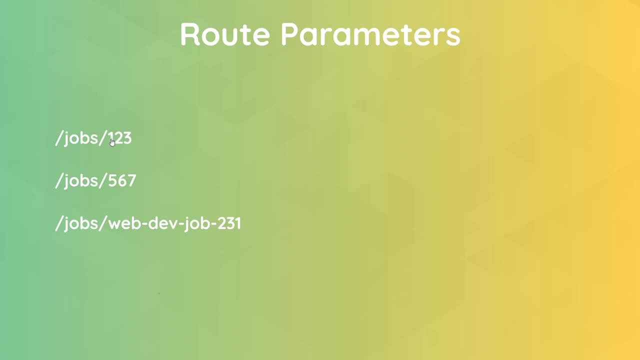 want to see the details of, for example, it could be forward slash 123 after jobs, or forward slash 567, where this number is the ID of the job that we want to see. or it could be something like forward slash web dev job 231, where this would be the ID, or, as it's otherwise known, the slug, so the last. 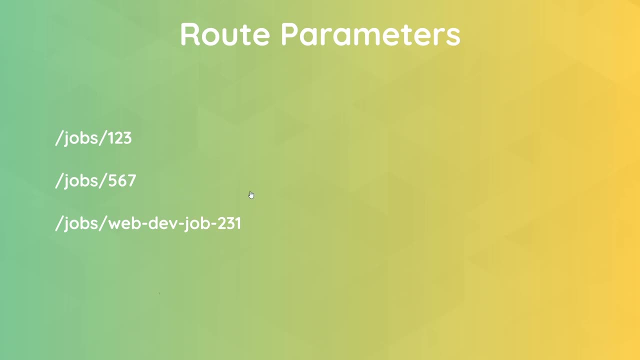 part of the route would be changeable, but it would always represent the ID of the job that we want to see, and then we'd show the details of that job in the details component, or the job details component in our case. now this changeable part of the route is known as. 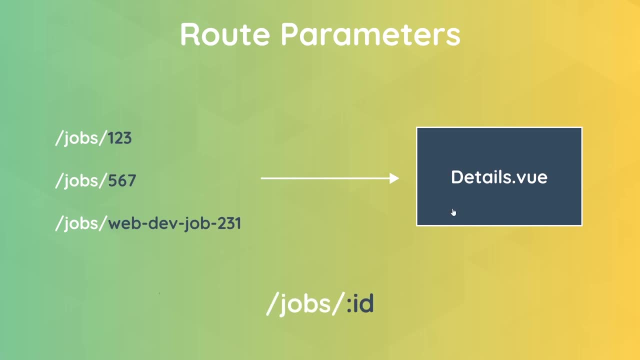 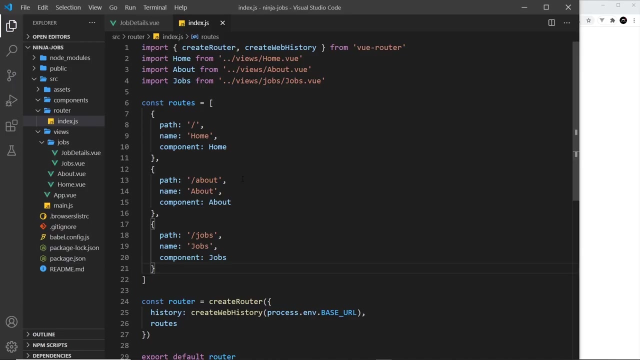 a route parameter and in view, we denote route parameters with a colon and then the parameter name. now the parameter name can be whatever you want, but a lot of the time you'll see it called ID in our application. the first thing we need to do is add in a route for the job details page, so I'm 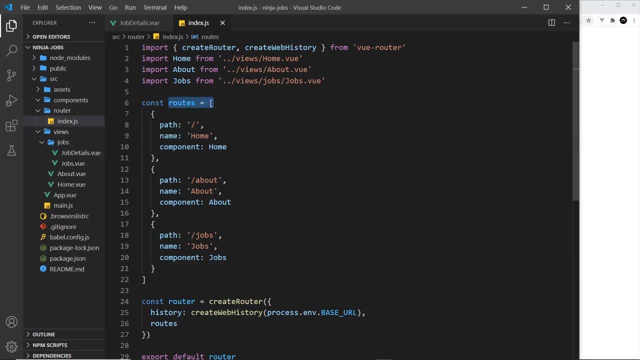 doing that. inside the router index file, inside the routes array at the bottom, create another object for this route. the path is going to be forward slash jobs and then it's forward slash the route parameter which I'm going to call ID. now, to create a route parameter, we do a colon. 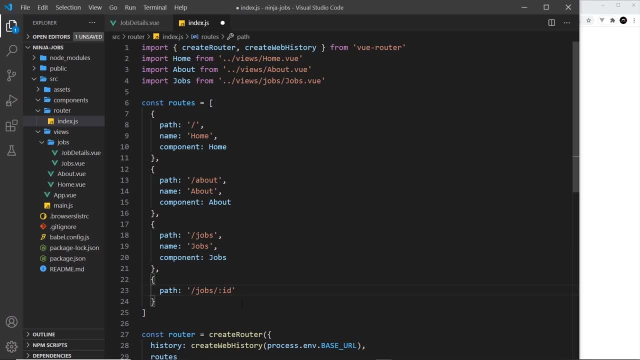 then the parameter name, whatever you want to call it- in our case it's going to be ID. then we need a property and this is going to be job details, and typically when I create a name it's always the same as the component name, most of the time anyway. and then we need a component and for 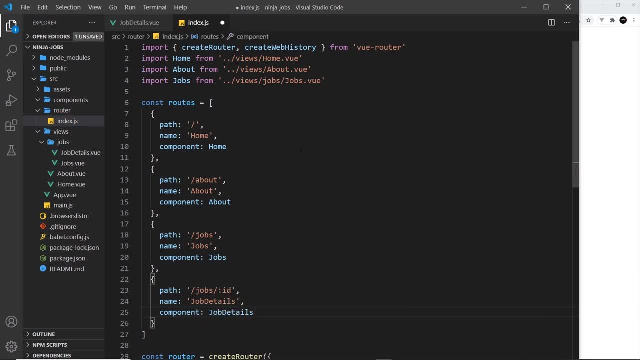 that it's the job details component. we need to also import that. so let me alt shift and press down to duplicate this and change this and this to job details. okay, so now, if we save that and go to this route, no matter what the ID is- it could be one, it could be 10, it could be Yoshi, it doesn't matter, it's. 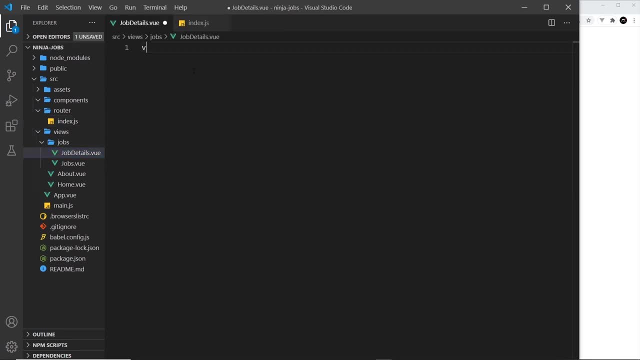 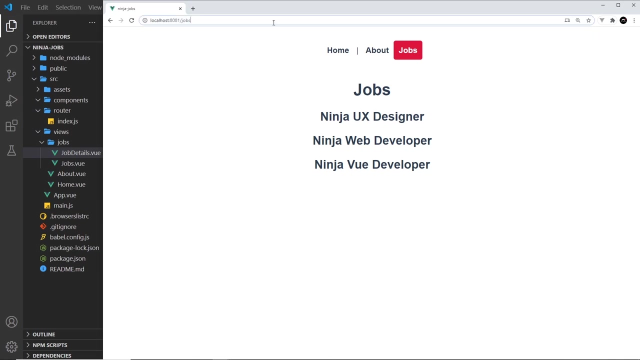 going to show this component, so let's go inside this component and flesh it out a little bit. all I'm going to do for now is an h1 which says job details page, like so, so that we know we've landed on it. so if we go to forward slash jobs, forward slash one, we should see the job details page, which. 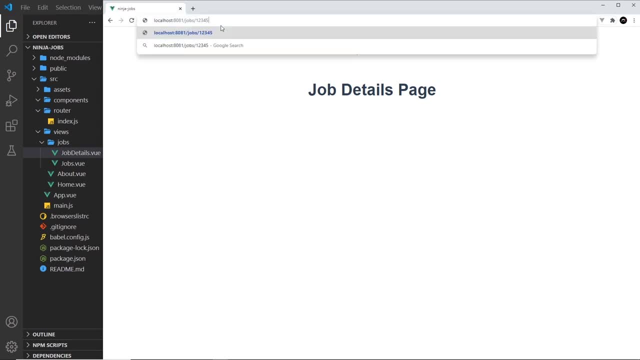 we do now this up here can be anything. it can be one, two, three, four, five, and we still get the job details page. or it could be Mario and we get the job details page. it doesn't matter what this value is. view recognizes that it follows the same. 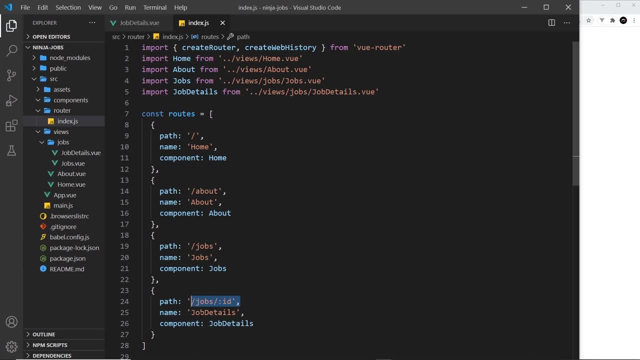 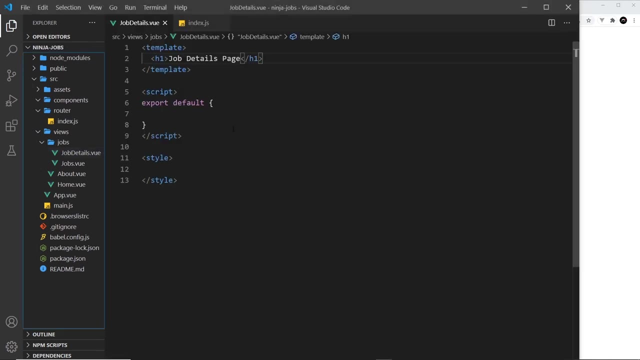 structure as this route down here, where the thing after the job is changeable because we said it can be right here, because this is a route parameter. okay, now it would be nice if that we could access whatever that parameter is right here- details component- because ultimately we want to show details about that particular job, so we need 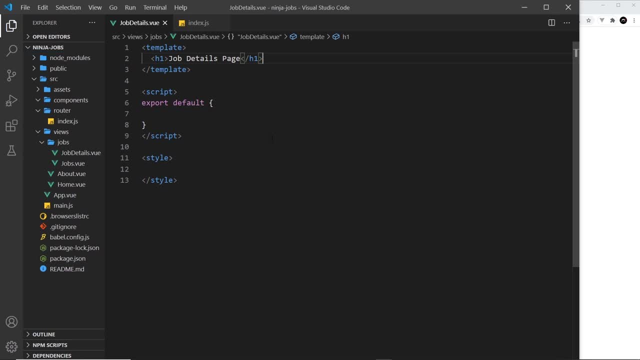 the id, so to access that, we can use the route object. so let me do a paragraph tag down here first of all, and i will say: the job id is and we're going to output a dynamic value, so curly braces, and we can say in here we want to use the route object, so it's dollar sign route and this: 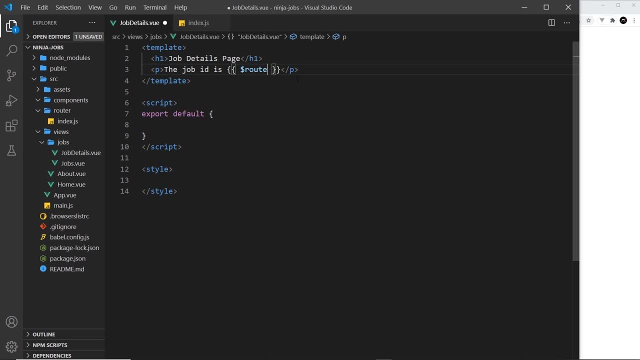 object contains information about the current route, including any route parameters like this. so i could say dot params to get the route parameters, but then i also need to say dot. whatever the route parameter is called, in our case it's id, so it would be dot id. but 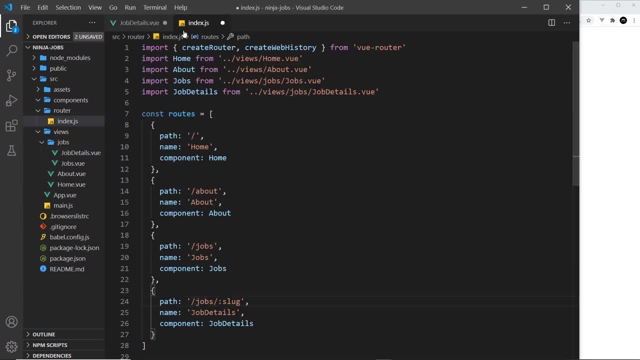 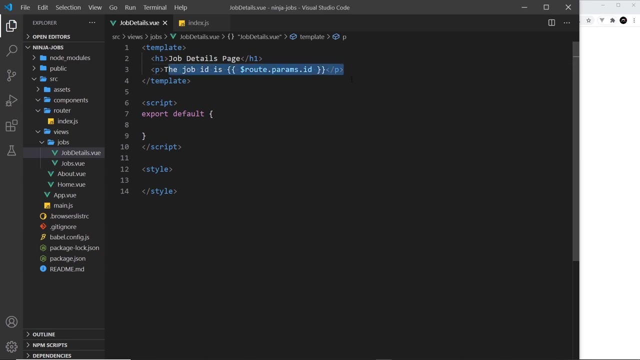 if the parameter was called something else, like slug, we would say dot slug here. so it's whatever the route parameter is called for that route. okay, so let's save it. hopefully now when we go to this route we're going to see the actual route parameter or the id of that job on the page. so let me refresh and we can see already. 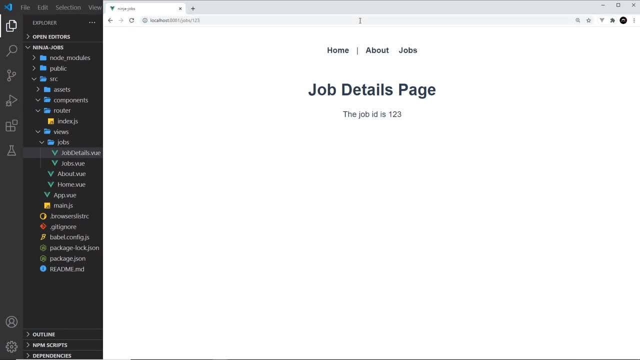 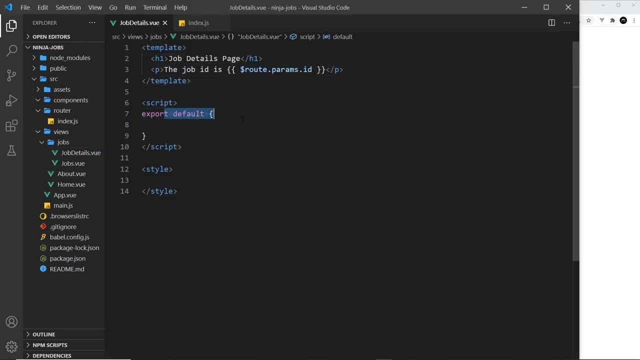 the job id is mario. if i change this to one two, three, the job id is one two, three. now we can also access this route object right here inside the component object as well. so let me do that. i'm going to set up our data function which returns an object, and inside here i'm going to say: i want 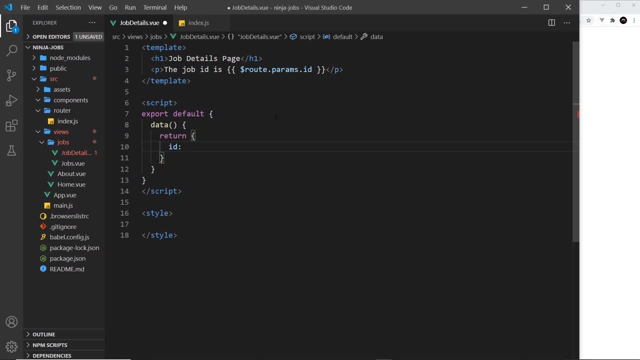 an id property to store the id of the current job. so we're going to get that from the route object. only this time, when we're inside the component object, we have to say this to reference the component object first, much like we do for data when we say this: dot, whatever the data. 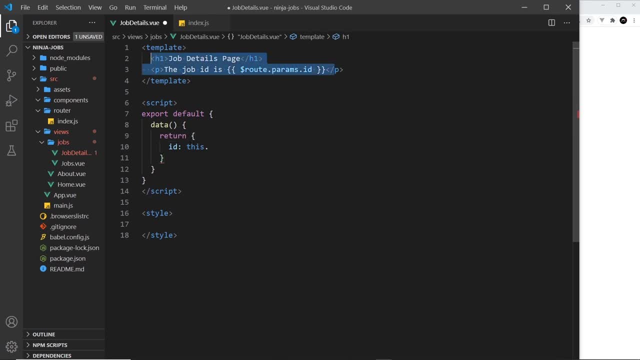 property is. we don't need to say this inside the template, but we always do inside the object of the component. so we say this: dot dollar sign route, and then dot params and then dot id. so i can now just output id right here to grab this property, which is the id from the route parameters. save that and it's going. 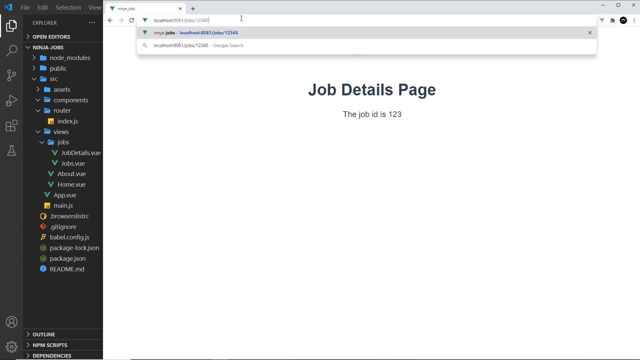 to do exactly the same thing: refresh, change this, and we see we get the id right here. so next up we're going to look at how to make dynamic router links which can pass route parameters, so that when we click on one of these jobs, it goes to the correct url at the top. for example, this one: 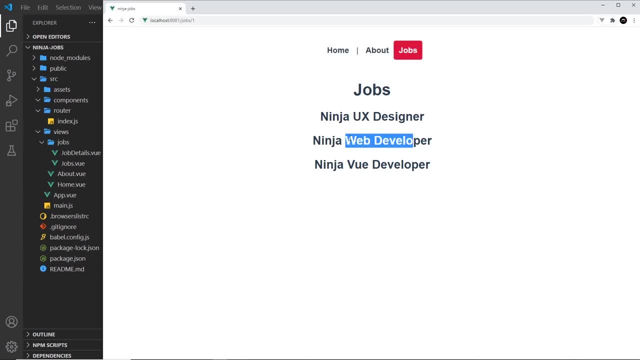 forward slash one. for the next one, forward slash two, etc. all right, then, so i'd like to make it so that, whenever we click on one of these jobs, it then redirects us to the url for that job, and it's going to be forward slash jobs, forward slash. 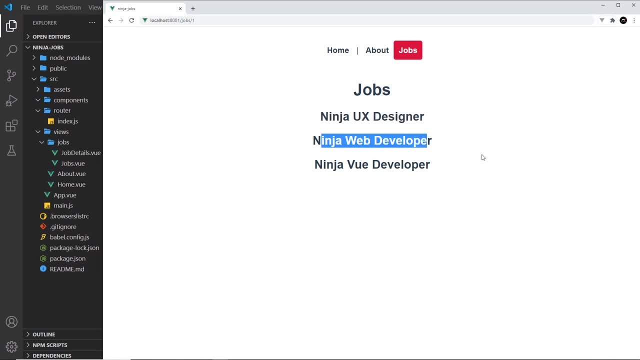 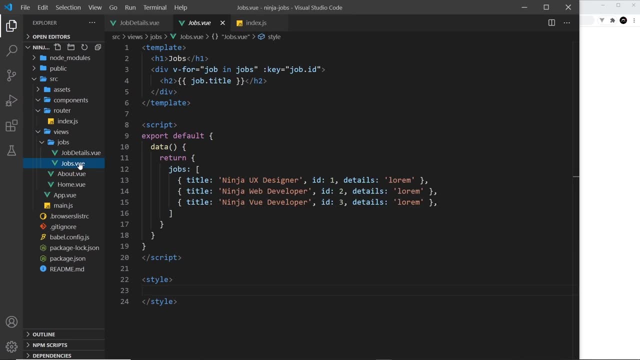 the id of that particular job so then we can see eventually the details of that job in the job details component. we're going to have to make up this route inside the jobs component where we output the h2. so i'm going to surround that in a router link. so let me cut this first of all. 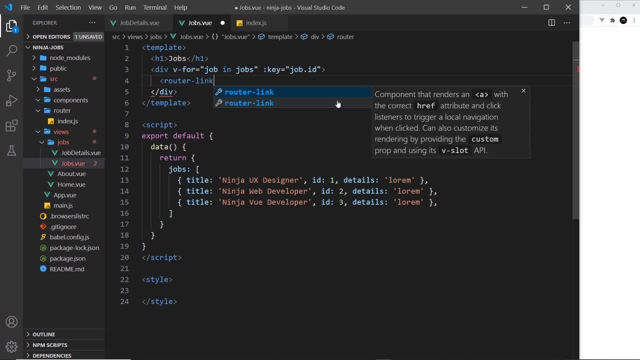 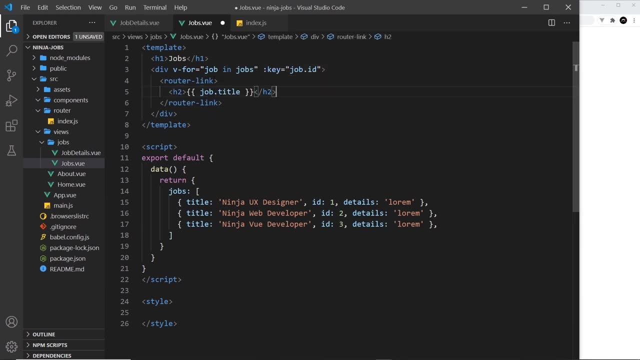 and then create a router link tag like so, and we're going to close that off as well, and then inside this i can place the h2 again. now we need a to attribute which is equal to something, and we're going to use the object inside here, so we'll data bind, so we can use an object. 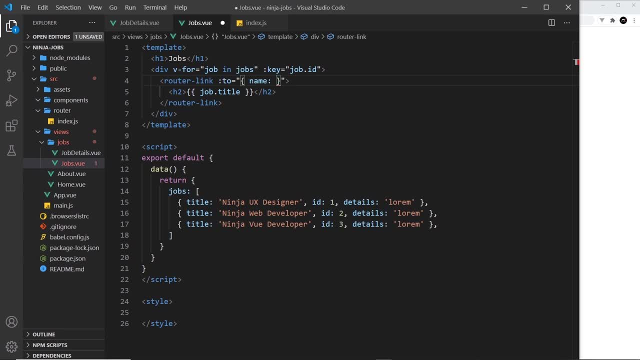 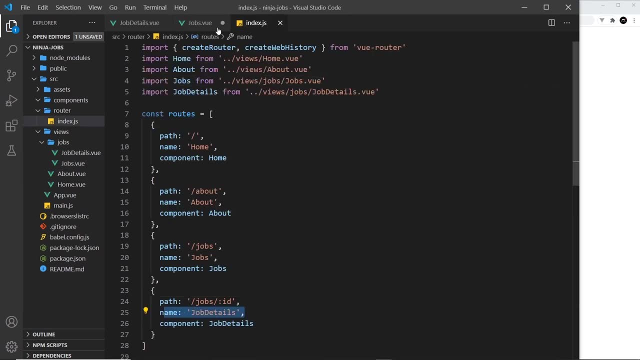 and the object has a name property. that's the name of the route we're going to and that, remember, is job details and remember the name is right here. so we're going to that route but we also want to pass through a route parameter, that is the id. 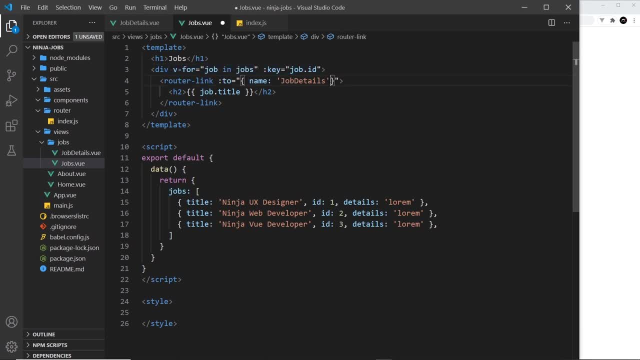 of the current job that we're iterating in this v4. now we can add parameters just by saying params and that is an object of key value pairs and each key is a parameter name. so we're going to pass through a parameter which is id. so that would be the key. 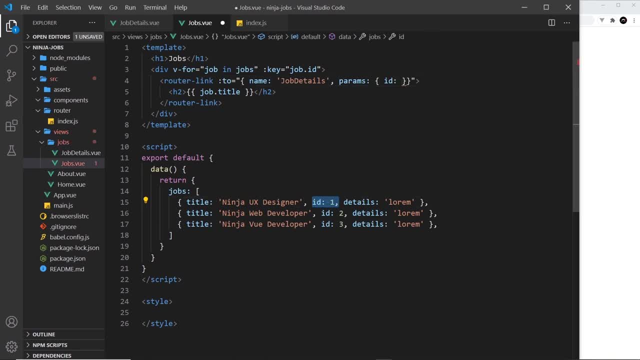 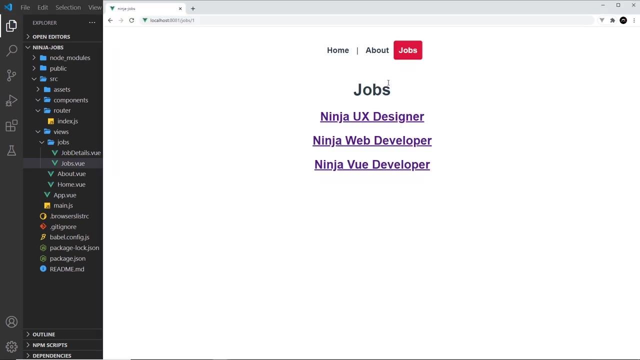 and then we pass the value. well, the id is on the job object right here. so we can just say: job which we have access to, dot id. so job, dot id, and that's it. that will now link to the correct route for that job. let me save this and show you. now we can see these are links, and if we 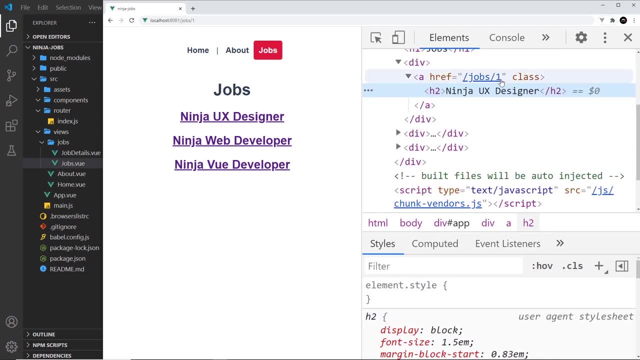 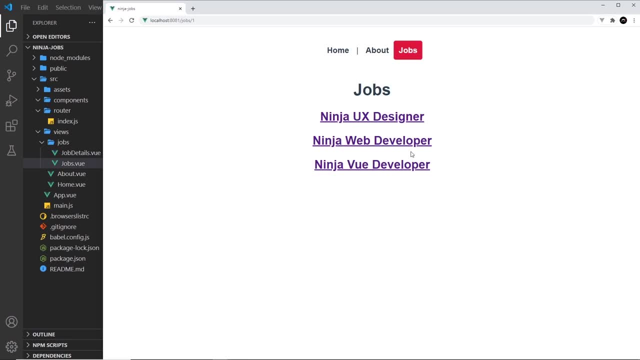 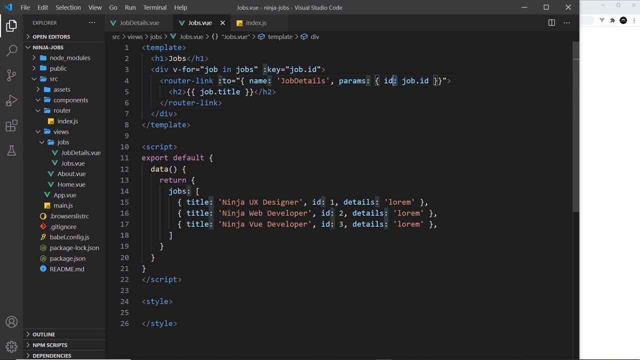 inspect each one, we should see that the first one goes to forward slash one, the second one goes to forward slash two and the third one to forward slash three. so we did that. we passed that route parameter to the url by using this params property. that's an object and then each key in that object. 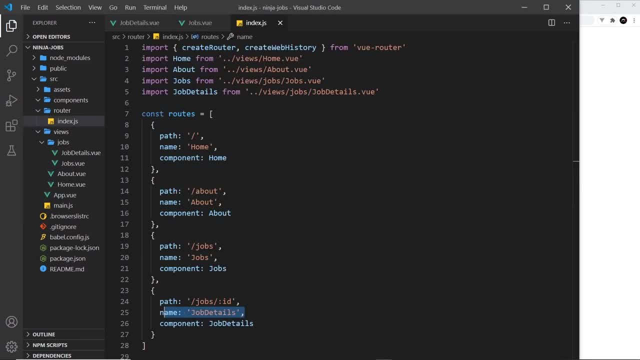 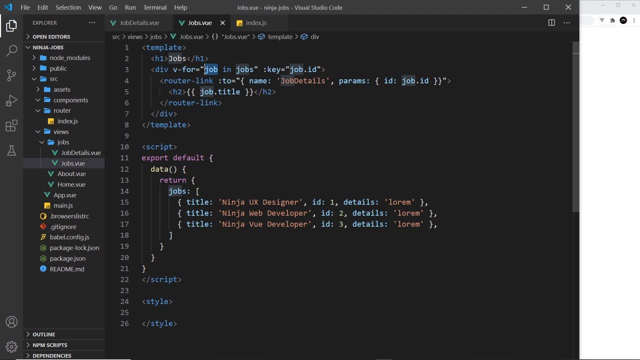 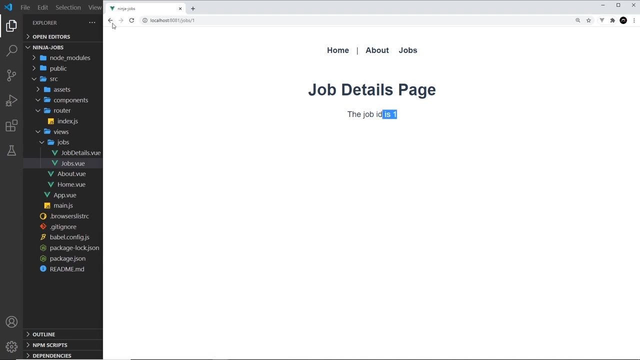 is a wrap parameter. we have an id wrap parameter- that's what we called it right here- and we've set a value of the id to be the id on the current job. so i hope that makes sense. so now we're sending that in and if we click on this we should be able to see the job. id is one. 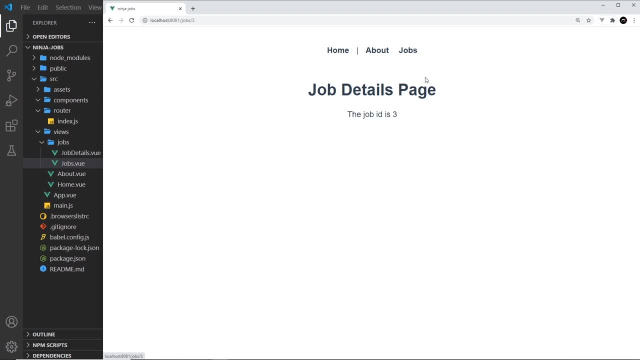 if we do a different one, let's refresh. the job id is three, so this is all working fine. we have access to the wrap parameter right here in the job details page and we can use that later on. but there's one more thing i want to show you. we can attach any route parameters to. 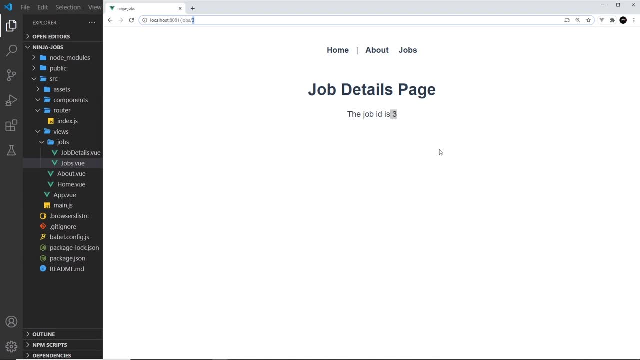 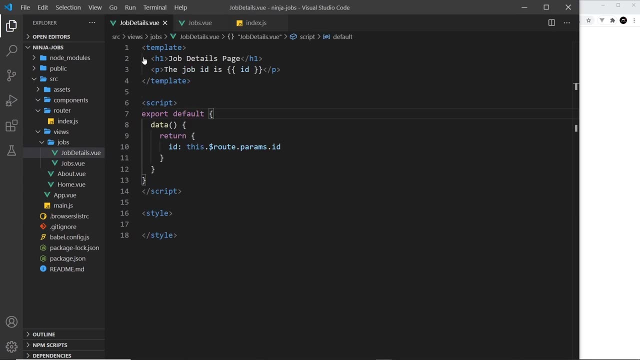 the props of the component we're linking to to make this a little bit easier. so, for example, the route parameter that we send in here, the id, i can accept as a prop inside job details, which is where we're linking to, so i could just say props and then inside here we want to accept the id prop. 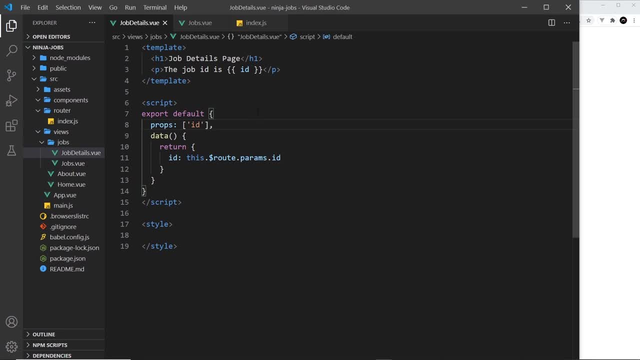 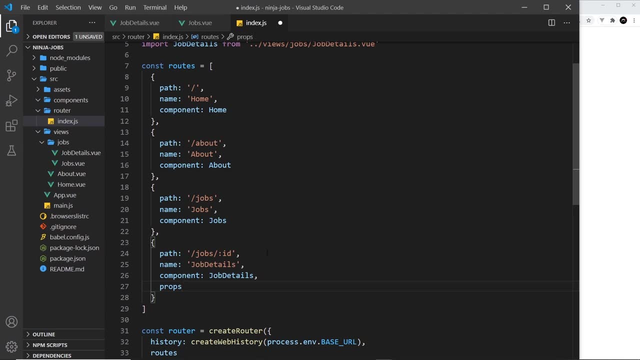 so this won't work straight out of the box like this. we have to do one more thing, and that is inside this route. for this component, we just add on a final props property and set that equal to true, and that means we can accept any route parameter as a prop, and that allows us to set very simply our route parameters as props and what. 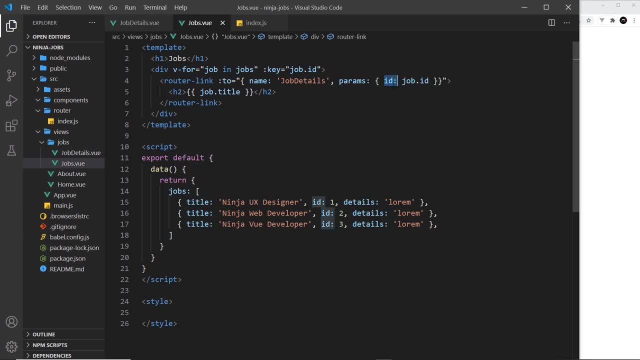 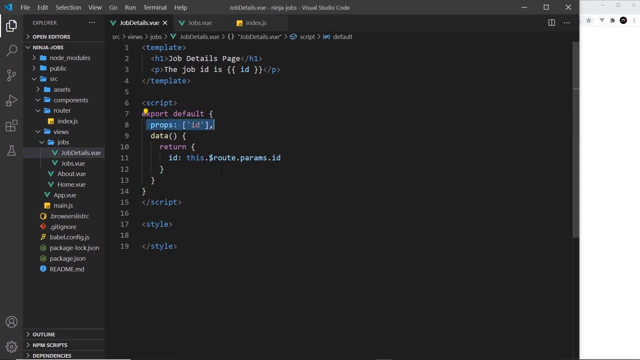 this will do is when we link to a specific component- in our case the job details component- and we pass through a parameter view will attach that parameter as a prop to that job details component. so now we can accept it as a prop and we don't need to do this anymore to get the id. so we 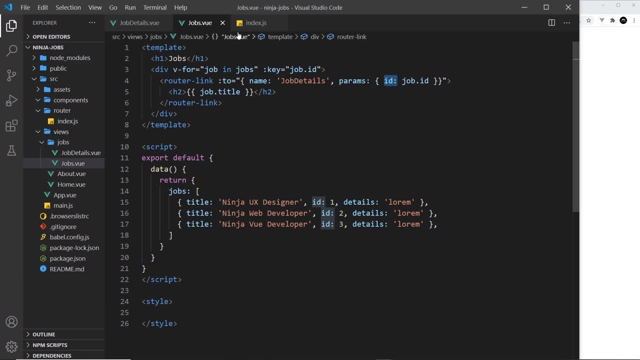 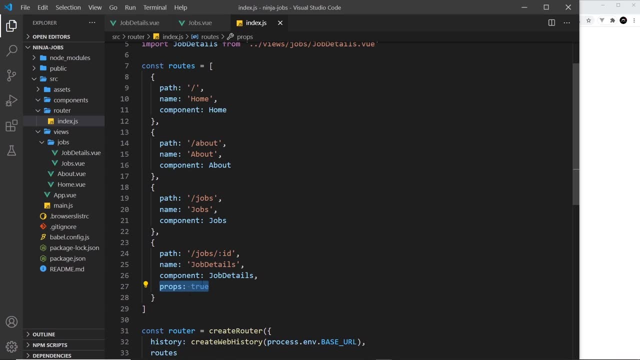 could comment that out, because we're now just accepting the parameter, the route parameter, as a said props, is true for this component route. if we didn't have this on, it wouldn't work. but since this is true, we're saying, okay, any route parameter that you send through when you link to this. 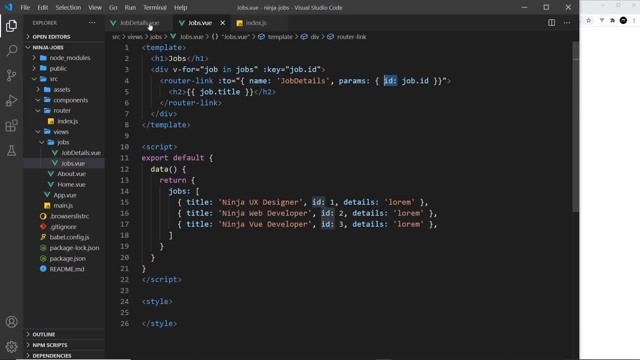 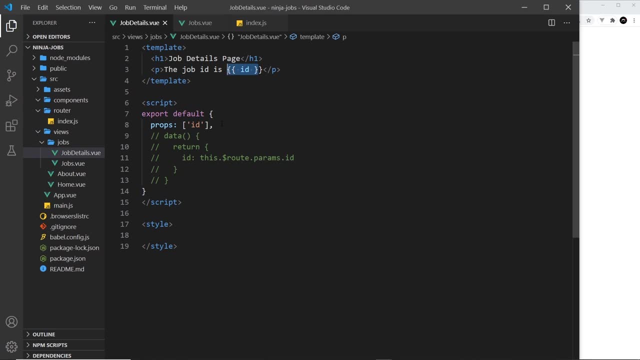 component like this: attach that wrap parameter as a prop to the component you're linking to so we accept it and we can output it right here, so you don't have to do this. this is just a nicer way of working with those wrap parameters and accepting them inside a component when we link. 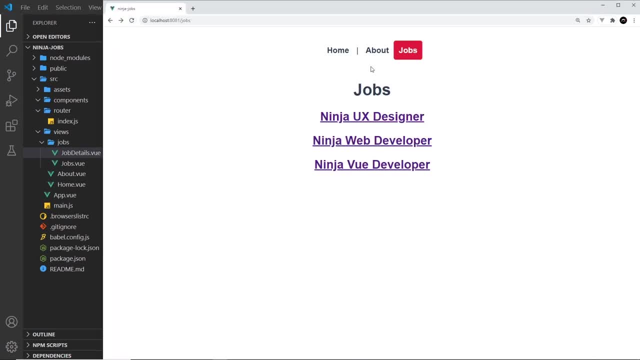 to it. so if we take a look over here, everything's still going to work exactly the same way. we go to one, and we see the route parameter. we go to two, we see it right here, Etc. so we'll probably see more of this kind of pattern in the future as well as we make more projects now. finally, I just want. 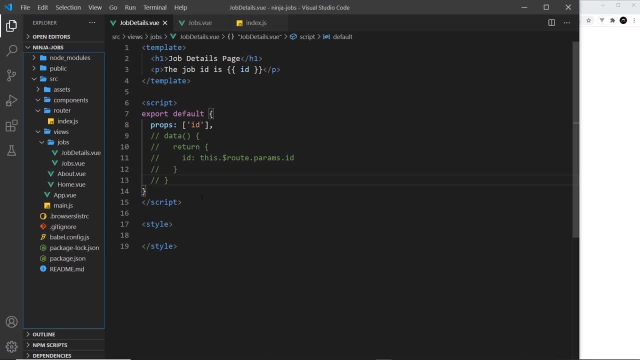 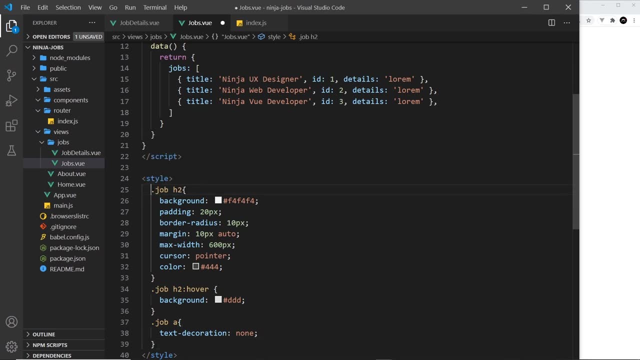 to style these links right here a little bit better. so let's do that inside the jobs component where we output them. I'm just going to paste in these styles so you can see we say job H2 first of all, and I don't think we actually have. 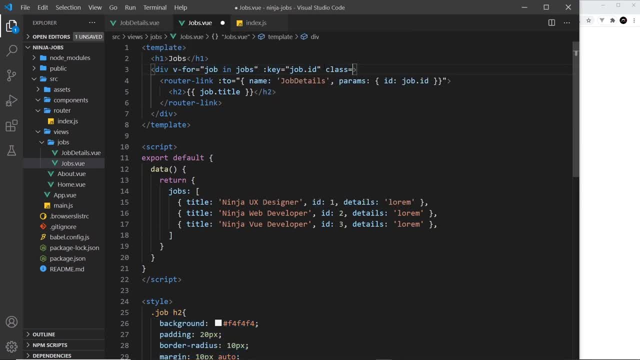 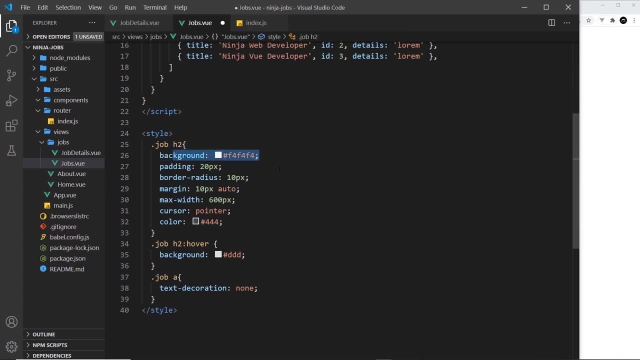 a class of job anywhere, so let's add that class on. so class is equal to job right here. so we go after this class and get the H2 inside it. we say we give this a background of a very light gray color bit of padding, some border radius, margin top and bottom and a max width. the cursor is pointer. 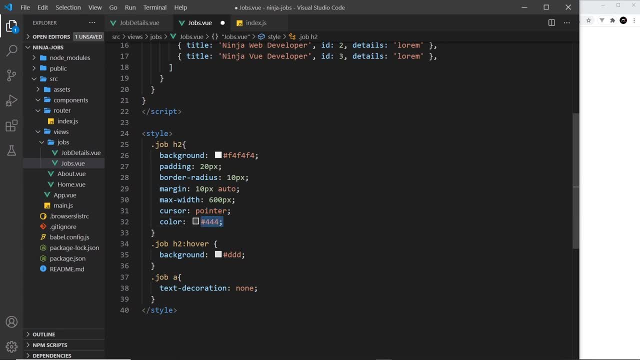 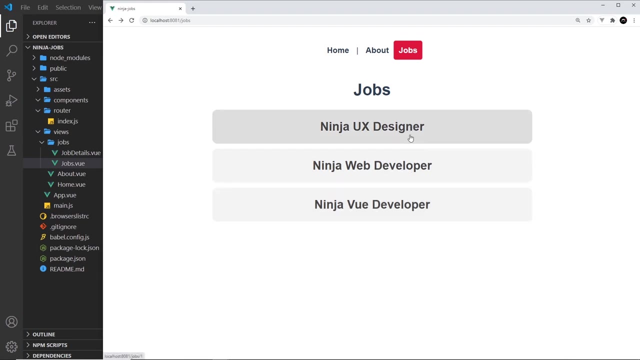 so we know we can click on it and the color of the text is a deep gray. when we hover over the H2, the background goes a slightly dark gray and the anchor tag is text decoration. not to remove the underline, save it and oops, let's go back. that looks, I think, a little bit better. awesome. so. 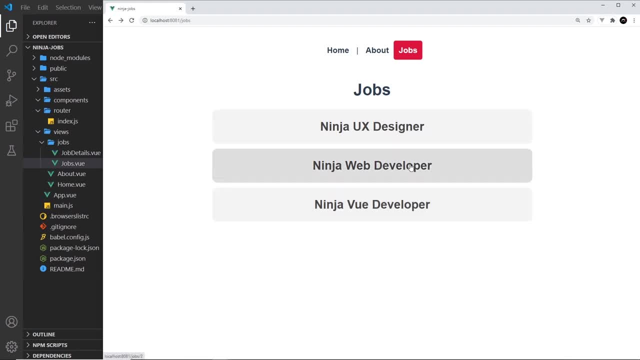 next up, I want to show you how to create a 404 page and also do redirects. so in this lecture, I want to show you two more things when it comes to the view router: first of all, how to do redirects and then, secondly, how to set up a. 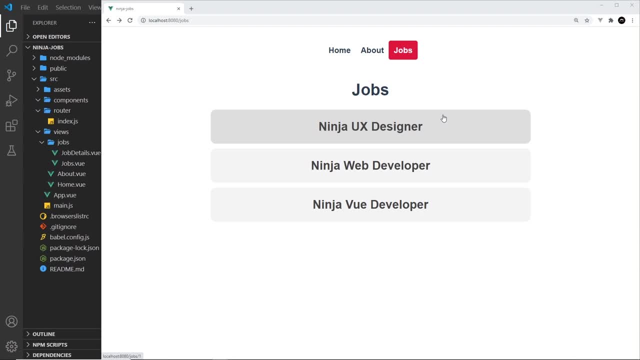 404 route for a 404 page if they go to some kind of route that doesn't exist. so first of all, the redirects. how do we set those up? say, for example, I want to redirect the path all jobs like this to just the jobs route, because maybe it used to be all jobs, but I changed that route. 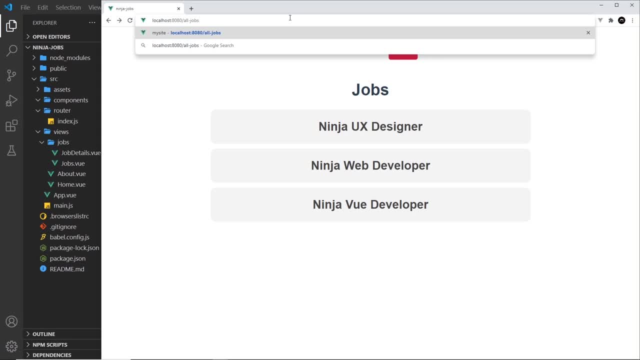 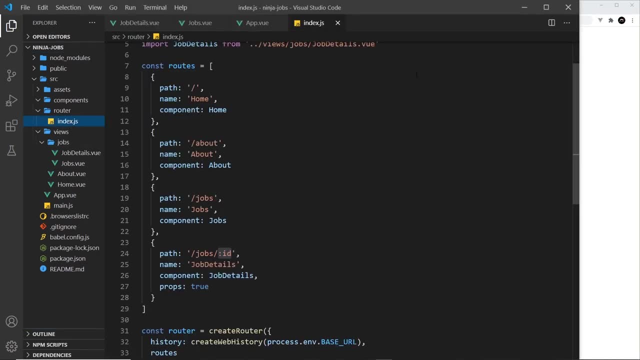 so I want to redirect anyone that goes to that old URL, the old route to the jobs component. well, that's simple to do. we need to go to our Index router file and then down here I'm gonna do the redirect. So we'll say redirect. 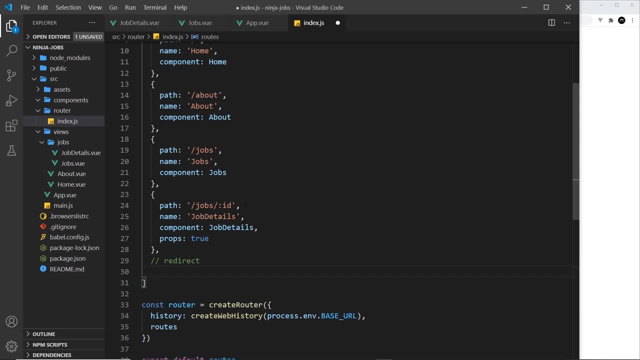 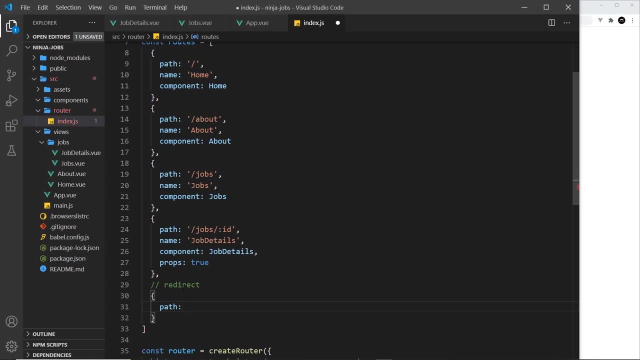 and, at the end of the day, this is just another route object that we place inside our routes array, and When we create this, the path is going to be whatever we redirecting from. so the old routes, in essence, And that would be all Jobs. so imagine, that's what the route used to be, But now we changed it. 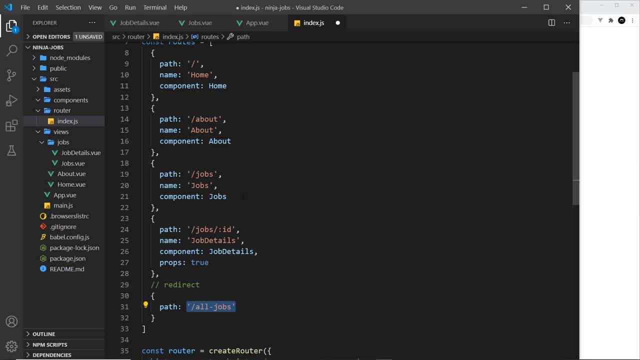 so it's just forward slash jobs. but we want to redirect this route now to this. all we need to do is add on a Redirect property and say where we want to redirect to. so, in our case, Forward slash jobs, and that's all there is to it. Now, if anyone goes to forward, slash all jobs. 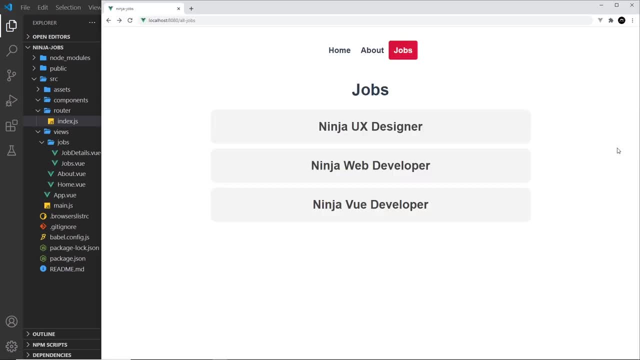 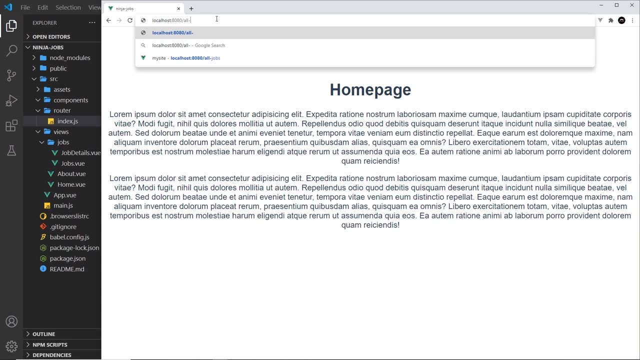 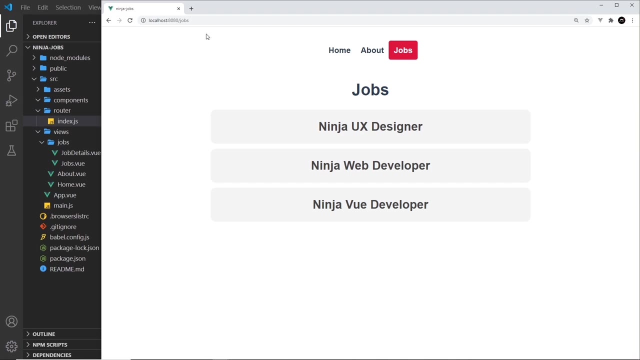 They'll get redirected to forward slash jobs. So let's try this out. I'm gonna press enter on this route And in fact let's go home first of all and then go to all hyphen jobs like: so Press this and you can see we get redirected instantly to forward slash jobs and we see the jobs component right here. 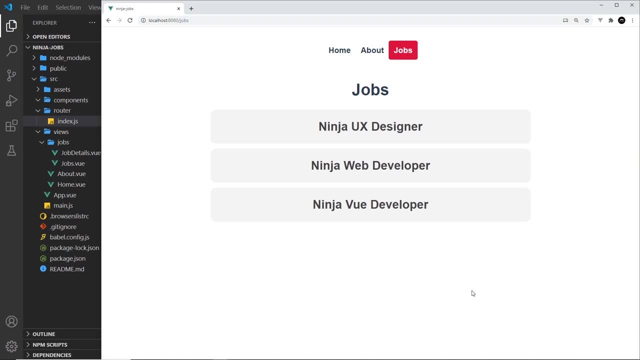 Okay, so that's the first thing I wanted to show you. The next thing I wanted to show you is how to create a catch-all route For any route that doesn't exist, so that we can show a 404 page. for example, If we were to go to forward slash ABC, then at the minute all we get is a blank page with the nav at the top. 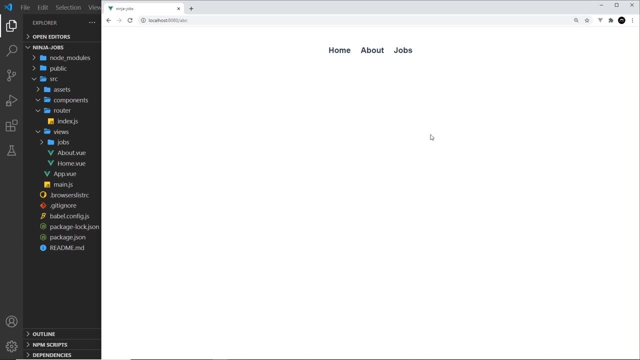 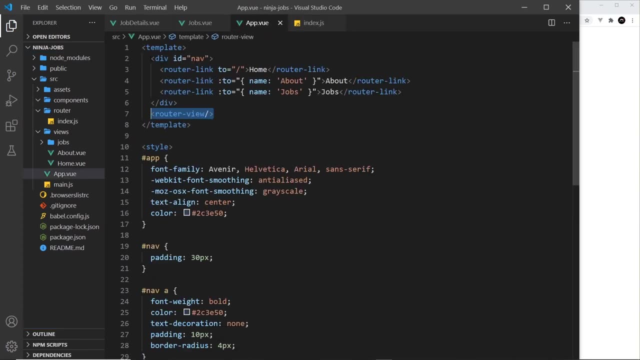 Nothing here to say that this page doesn't exist, It's just blank. So we get the nav because, remember, the nav shows on every route, Regardless of the route, because inside the root component the nav is right here, It's not inside the route of you. 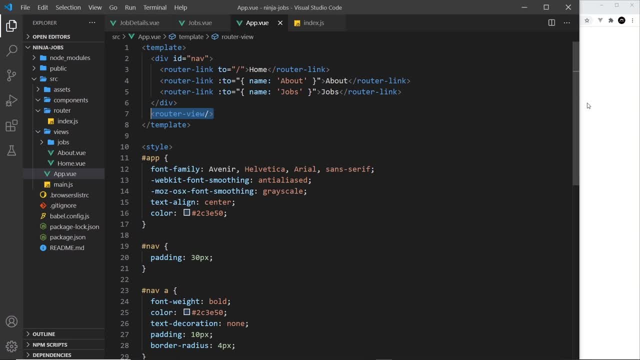 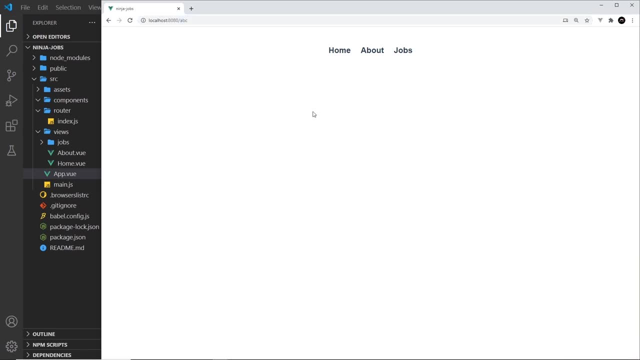 This is the only bit that changes dependent on the routes, So this thing right here is not very helpful. instead, when a user goes to a route that doesn't exist, like this, I'd like to show some kind of 404 page or not, found page. So the first thing I'm going to do is create a view for that. 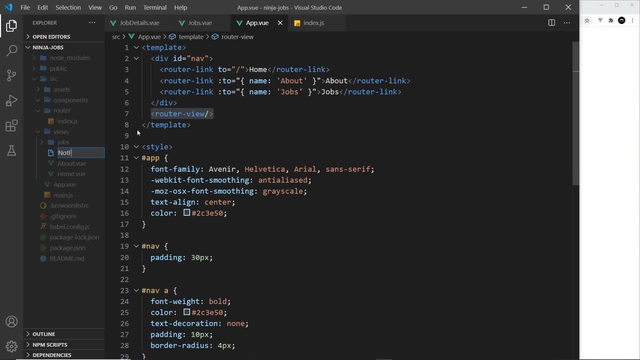 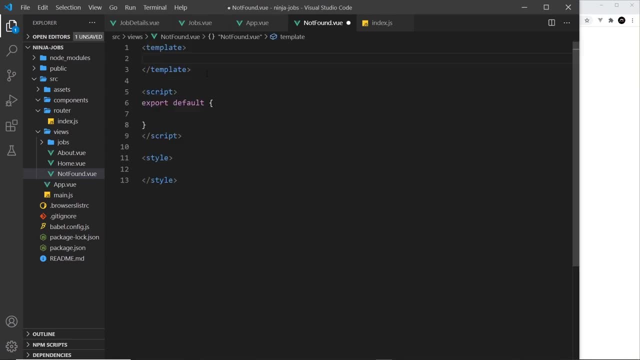 So going to views a new file and I'm going to call this Not found, but you can call it what you want, It doesn't have to be called this. and then I'm going to Boilerplate this component and create a template. So first of all we'll do an h2 to say page, or rather 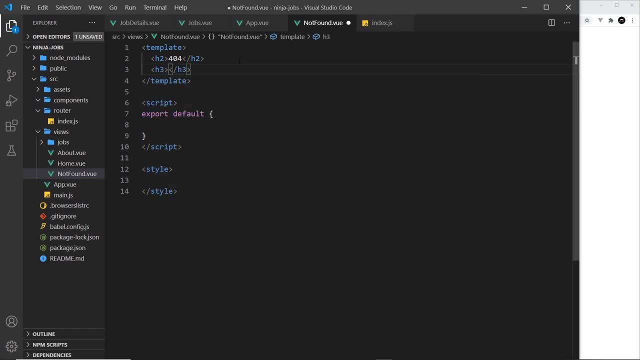 We'll say 404 here and then underneath we'll do an h3 to say page not found. Okay, so I'd like to show this component when we go to any route that doesn't exist And in fact we don't need the script or the style so we can get rid of those. 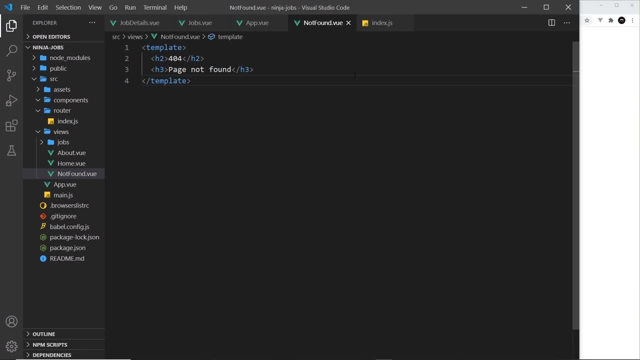 So how do we do this? How do we implement A 404 catch all page or rounds? Well, we go to our routes file, which is this thing over here, and we need to add on another route object down here. So let me do a comment to say catch all. 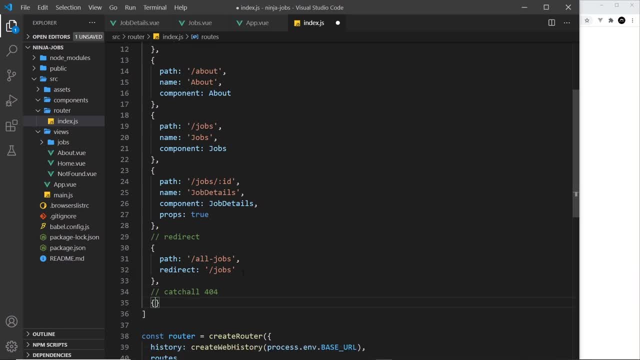 404 and then below that we'll do our route object and this time the path is going to be something very specific. It's going to be forward slash, then colon to denote a route parameter, and it has to be catch all, exactly like this camel case with a capital a, and then it looks like a function because we're using parentheses. 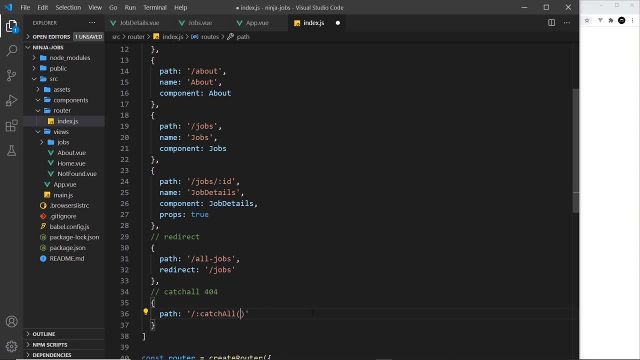 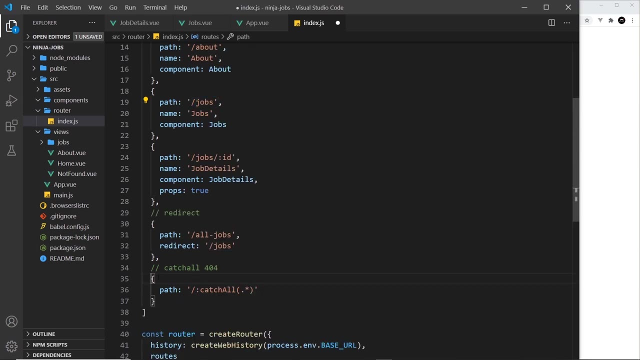 but really this is just a reg X pattern and Inside that we say dot and asterix and that will catch any route that is not caught by any of these other route objects. So if we try to go to something that doesn't match any of these, then this route object will catch that and we can do something. 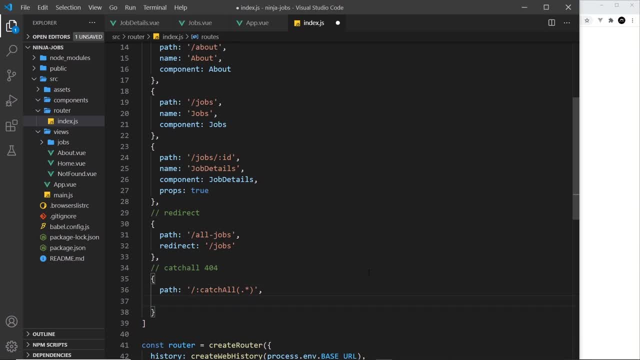 With that route. So, for example, I could say: Go to a specific component- First of all, I'm going to give this a name, though, and that will be not Found, and then under that we'll say: the component that we want to use is the one we just created, not found now. 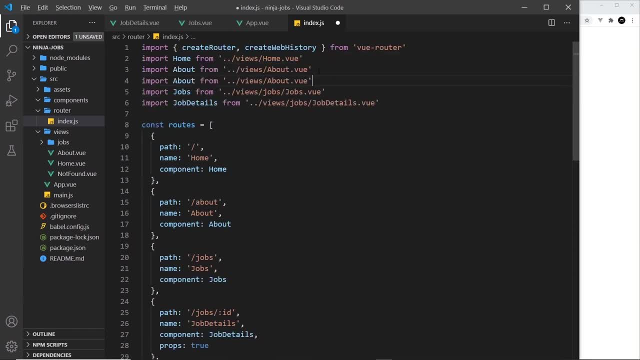 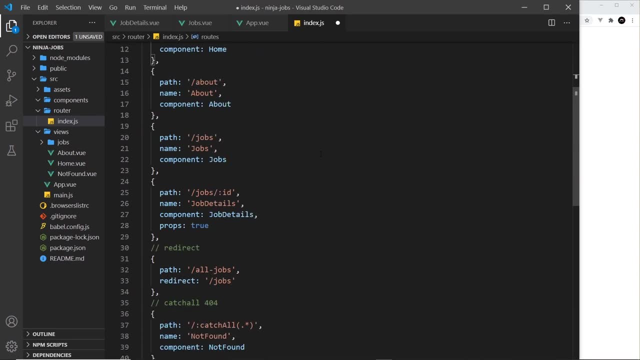 We need to import that, so I'm going to just duplicate this one right here and change about to Not found like so Okay. So now if we go to any route that doesn't exist, then it's going to catch that route and we're going to show this component. 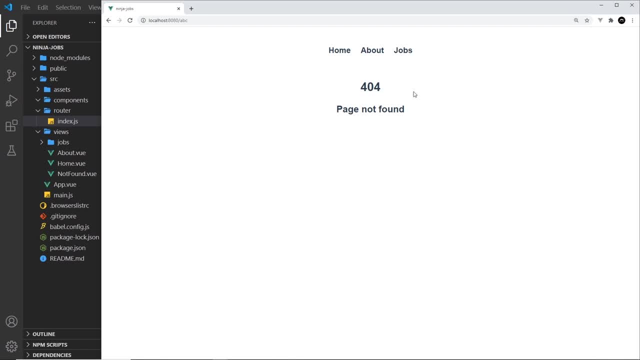 so Let me say this, and we can see already: we see 404 page not found. if we go to something else that doesn't exist, For example forward slash Yoshi, we get that as well. But if we go to these current routes that do exist, we get the relevant component for those routes. now in a real project, 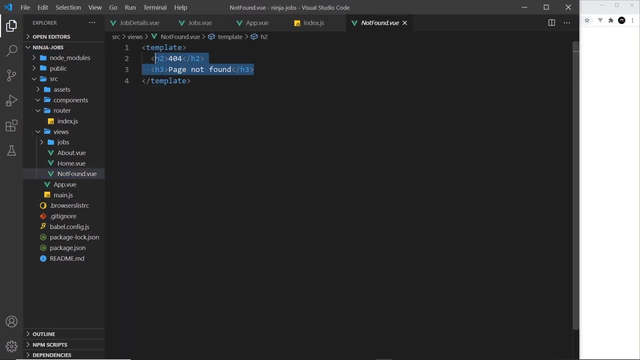 You'd probably make your 404 page a little bit better than this and give the user a bit more information, Maybe some links to navigate around the other parts of the website, but for now I just wanted to demonstrate how we can serve up a 404 page. 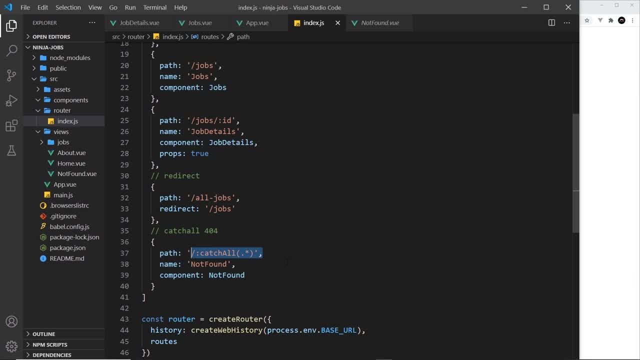 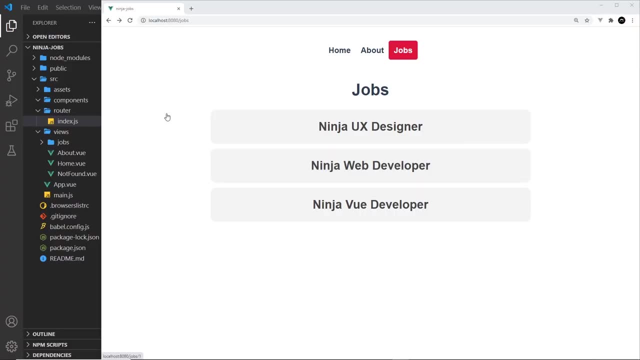 Using this thing right here, this catch-all regular expression. Now, when we use the view router in view applications, It uses the web history API and that means that we can go forward and backwards Using these buttons in the browser through the history of our journey in the website, if you like. now we can tap into that functionality. 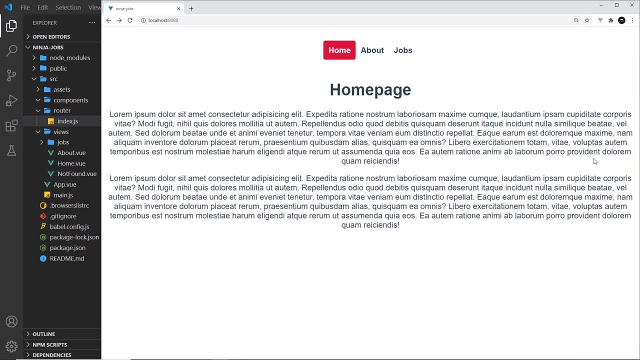 programmatically in view applications to send the user back a page or forward a page through the history, And also we can programmatically Redirect them to another route by pushing a new item onto the history. So I'm going to show you how to do all of that now. 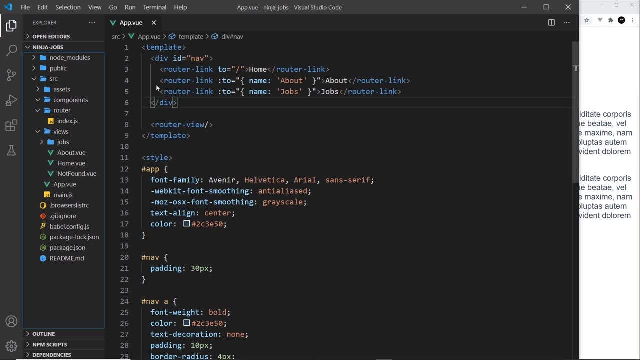 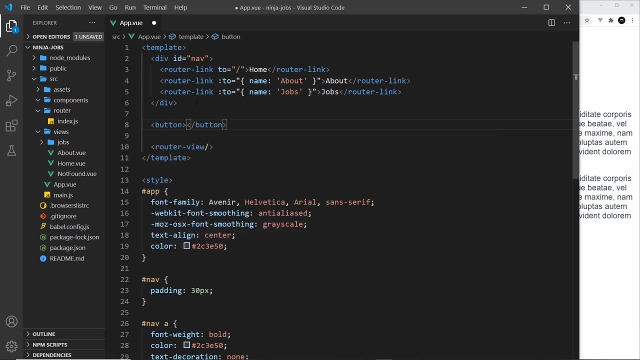 So to demo this, I'm going to go to our root component, app dot view, and I'm going to create three buttons below the nav But above router view. so let me create those. first of all, button button button, and inside the first one we will say we want to redirect the user and 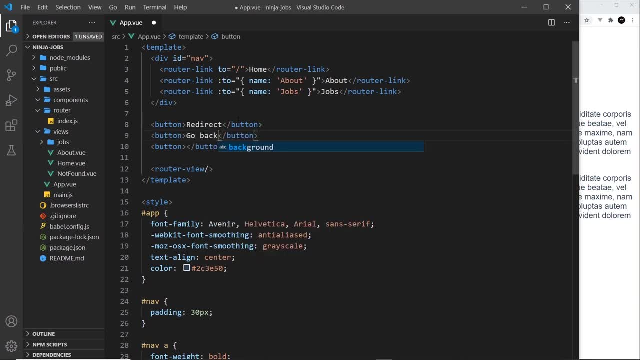 then the second one will be Go back a page and the third one will be go forward a page. So pretty self-explanatory. when they click this, I want to perform a redirect. when they click this, I want to go back a page through the history, and this won't go forward a page through the history. 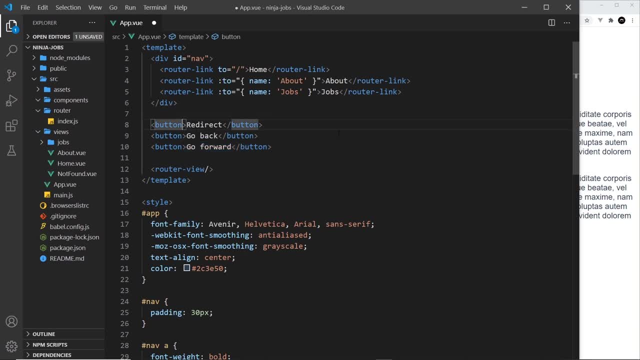 Now we need to attach click events to each one of these and apply handlers to each one as well. So let's do that. I'm going to say at click is equal to a function. now, We've not created any of these methods yet on our component object, And in fact we don't even have a component object. 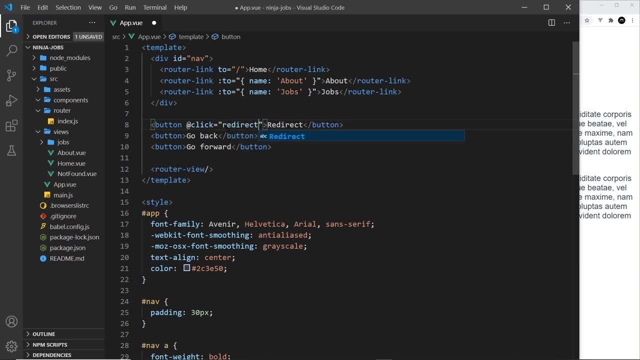 Yeah, but don't worry, We'll create those in a second. So this one will be called redirect. the next one down here, at: click is equal to back, and then down here, And click is equal to surprise, surprise, Forward. All right, So now we need to create these methods, and we need to create them inside a script tag. 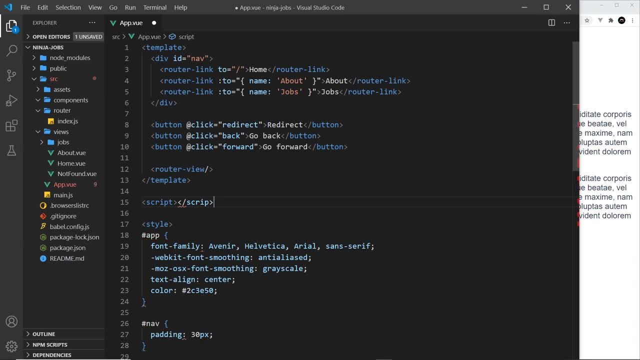 because we want our component object and That goes inside a script tag. in here We need to export Defaults, because that's always what we do when we have a component object inside a view file. And then we need our methods property where we can make these methods. The first one is called redirect. 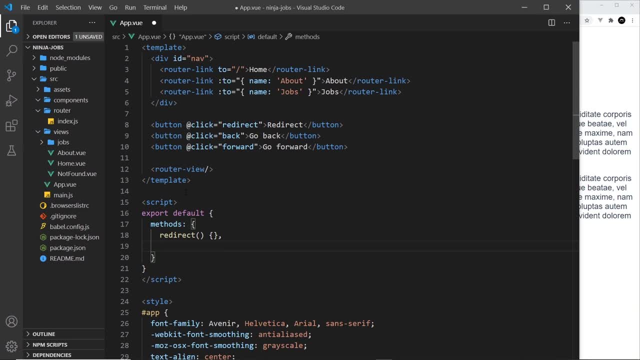 like so, and then after that we need one called back, and Then after that we need one called forward. Alright, so we have these three different functions Now. I just want to preview this to see what it looks like, and, yeah, They don't look great. 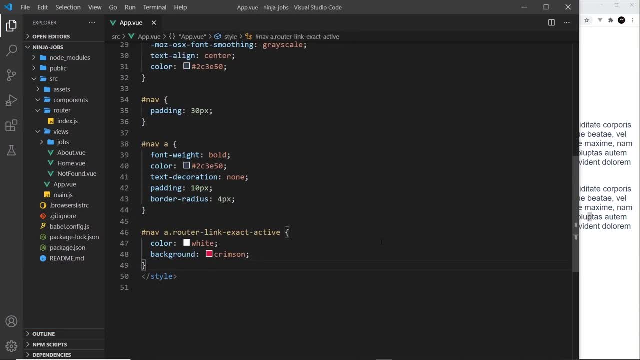 I'm just going to apply a couple of styles to it, So let me just paste these in. you can see, dead simple. We give each one a bit of margin to the left and right, a bit of padding, no border and a border radius. So we basically just spread these out a little bit So they look a little nicer. 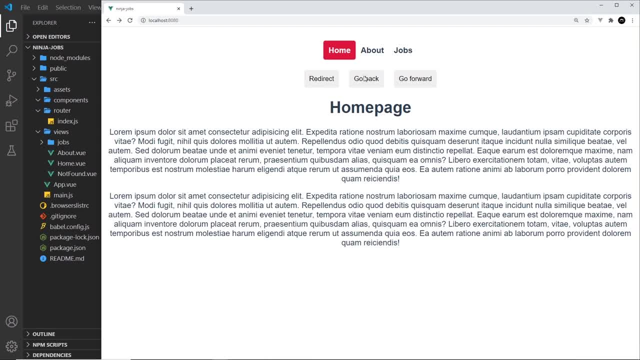 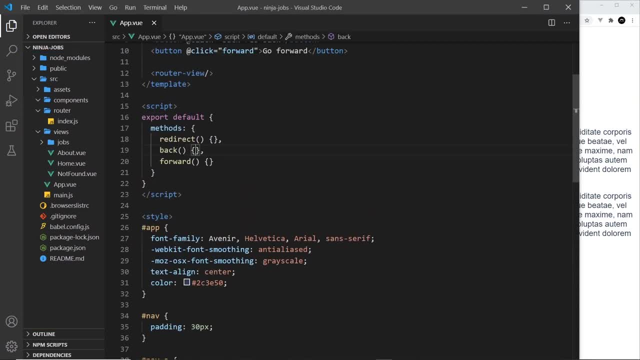 Alright. so then, when I click on the go back one, I want to go back through the history, So let's do that one first of all. Now, the way we do this is by saying this to reference the component instance, and then we can say: dollar sign. 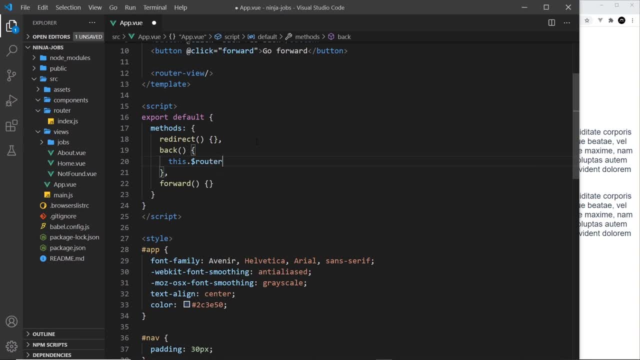 router Now, before we used dollar sign route to get the route parameter. don't confuse these two. We use the dollar sign route to get information about the current route up here. We use the router when we want to do something like move them around, and that's what we're doing. 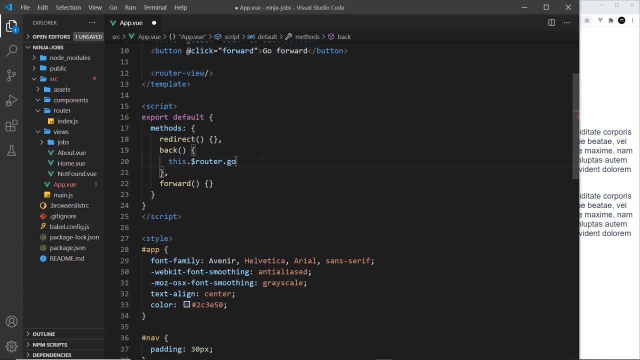 so we use the router and then we can use a method called go, and In here we can pass through either a minus number or a plus number. if we pass through a Minus number like minus one, it means go back through the history. So let me just demonstrate this. 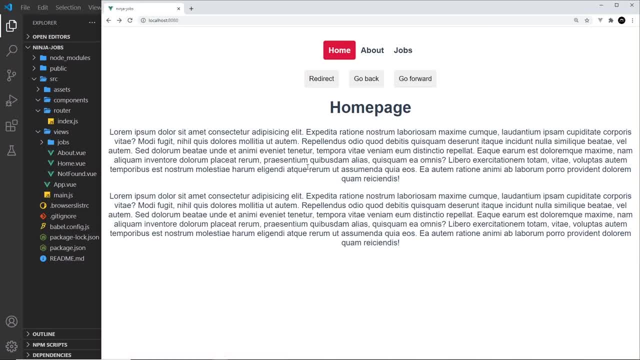 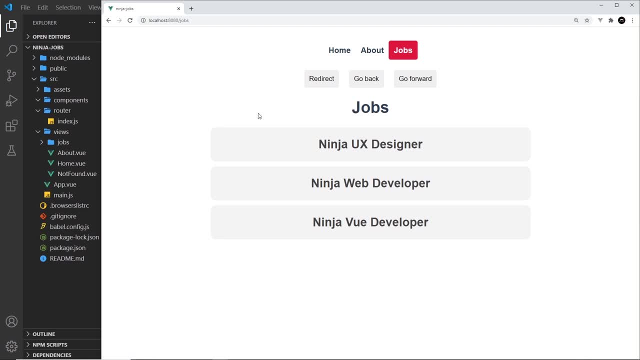 I'm gonna refresh on the home page to begin at the start over here. So we're on the home, then I'm gonna go to about, then I'm gonna go to jobs. Now if I click the go back button, it should go to about and it does. and if I click it again, 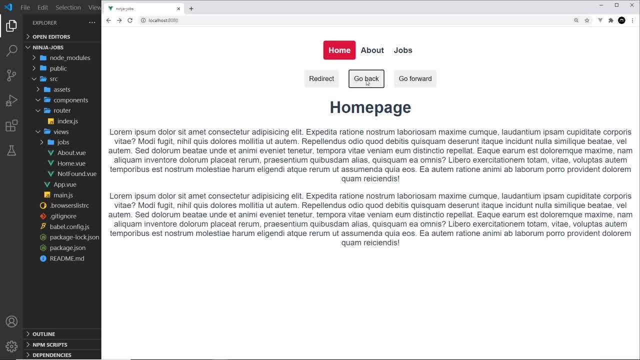 It should go to home and it does. and if I try to do it again, It's gonna go back to what we were on before that. So that's us going back through The history one step at a time. now this can be any number you want, for example: 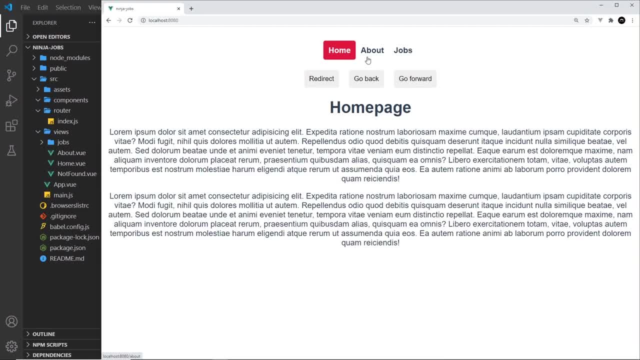 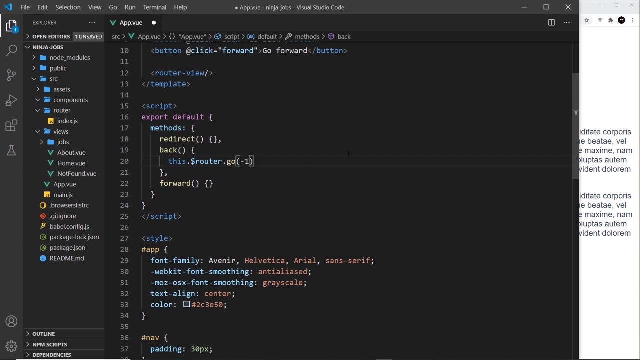 Minus two. now if I go forward to- so I'm currently on home- then about then jobs And then if I click, go back, it should go back one, two back to home, like that. So this is how many steps you want to go back through the history. now I'm just gonna leave it at minus one. 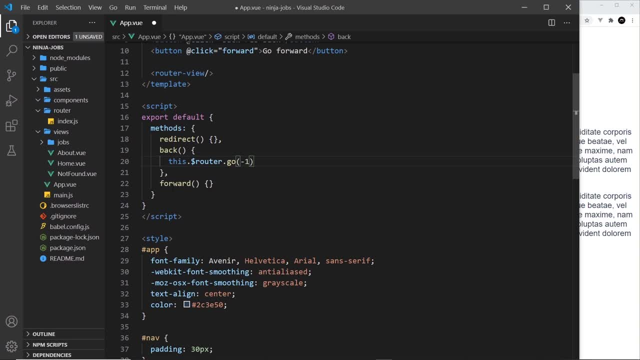 So remember, minus is go back through the history. Now The opposite is true for forward again. We say this dot router, and Then we say dots, go to use the same method. this time It's a plus number. now We don't have to write plus, we just write the number, because it's automatically a plus number. 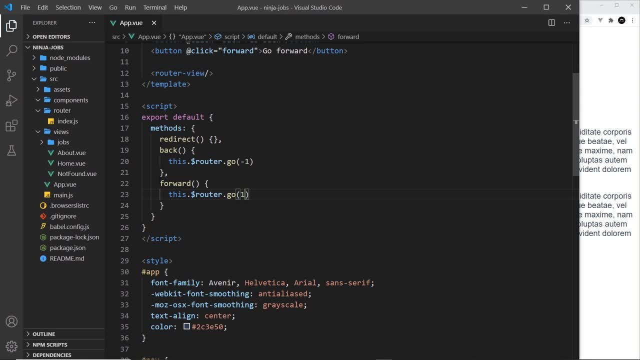 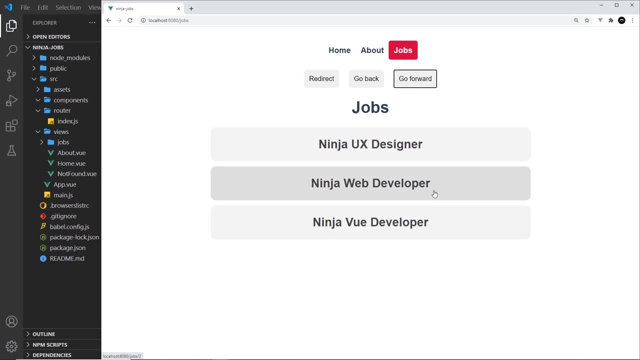 So I could go forward by one or two, doesn't really matter now if we tried this out. if I say go forward, Then it goes to about. if I say go forward, it goes to jobs. All right. now if I try to do go forward again, It's not going to go anywhere, because that's as far as we got. we didn't go any further because from then we would.